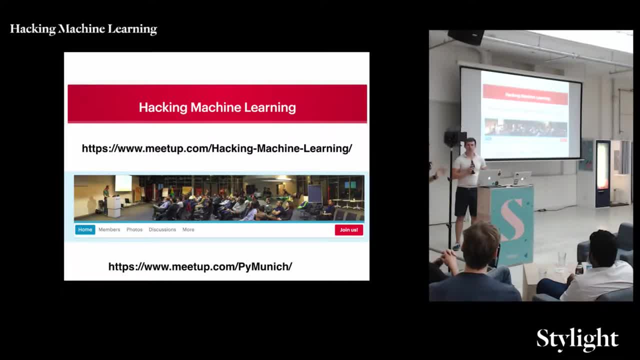 Okay, so I'm super happy to welcome you here together with Sergei. Don't be surprised about two meetups together, because it's about machine learning, right? Machine learning group. and what is the language mostly used in machine learning? Try to guess it, obviously. 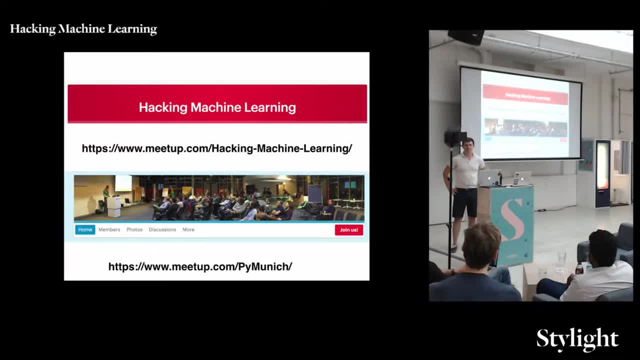 So, yeah, I'm super happy that we found today such awesome speakers, and they will be giving great talks today. We will chat more during the break, so I would suggest that we just jump right away to the talks. yeah, Yeah. 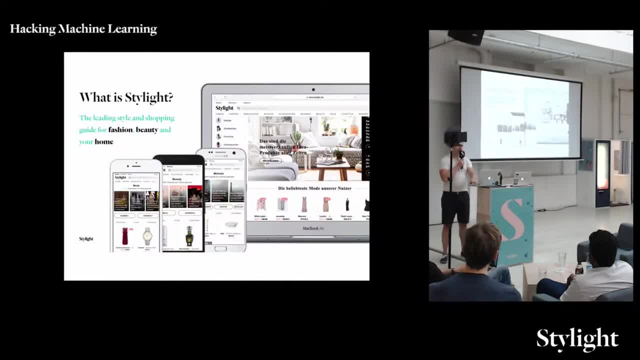 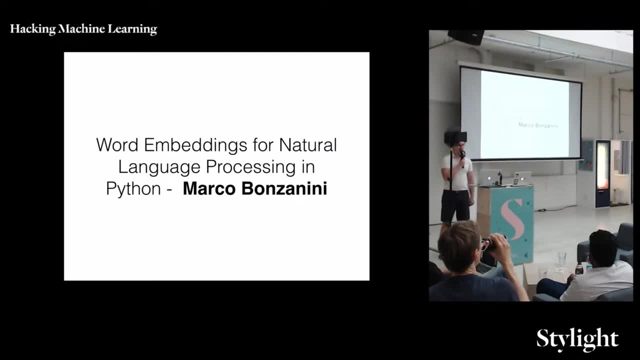 Okay, cool, So just like agenda-wise. I mean, it's hosted by Stylight and you can ask me what is the company about? So we have two talks today. One is like about word embeddings from Marco and after we might have like a short break like I don't know if you need to go to the toilet. 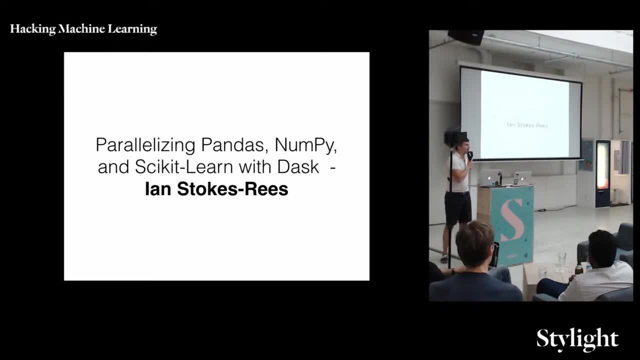 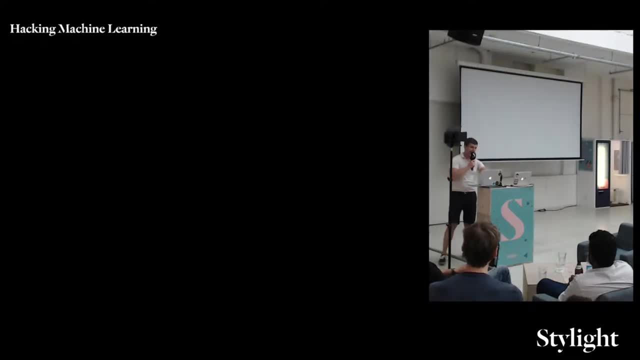 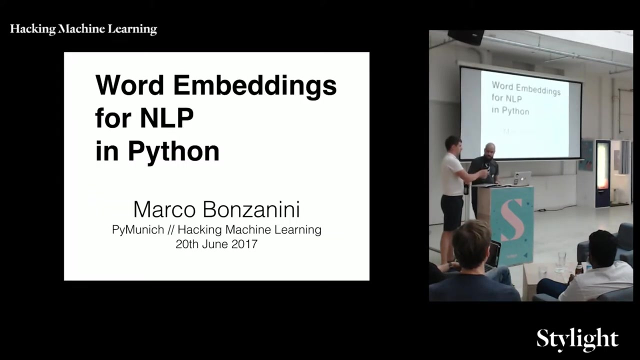 And we can have like about Dusk and how to parallelize your Python and make it like super awesome. Yes, and with that I'm handing over to Marco, So please welcome Woo. Okay, thank you. 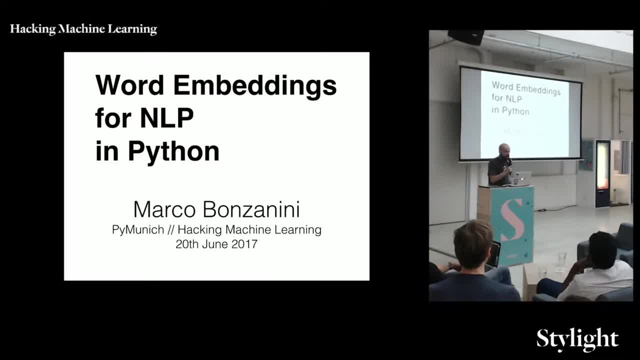 Thank you, Sergei and Anton, for having me and thanks everybody for being here in numbers. So this talk is about natural language processing and, in particular, word embeddings, which are a family of algorithms that are kind of gaining some traction right now. 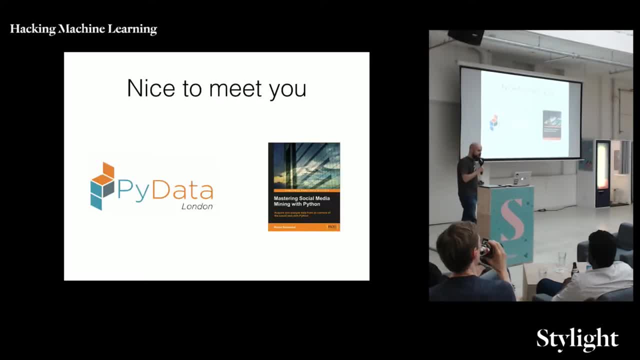 A couple of words about me. So I'm based in London. I co-organize the PyData London meetup and conference, so we run a monthly meetup kind of similar setting: a couple of talks, nice people, a few beers and so on. 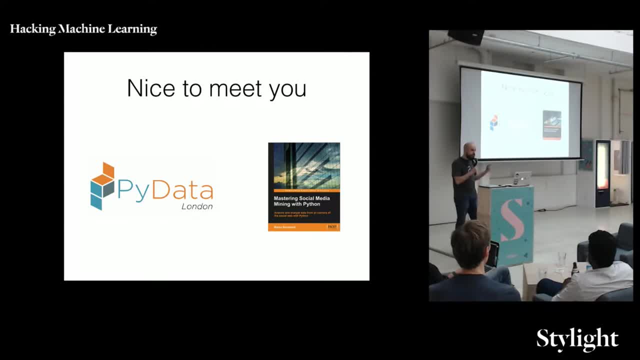 And we also run our annual conference. It was a Back in May, also in London, and on the right side you see some work that I've done. This was a book published last year on data mining for social media, So the job title is data scientist, whatever that means, and in particular, I try to focus on text analytics. 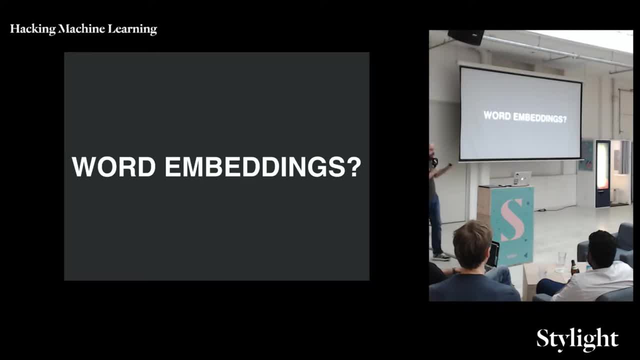 So word embeddings. the structure of the talk will be kind of an informal introduction on word embeddings, first what they are, what we want from them, And then a little bit of theory, but not too much. This is meant to be really an introduction. so if there are machine learning experts in the room maybe you will not learn too much on the machine learning side, but it's more on the linguistic intuition. 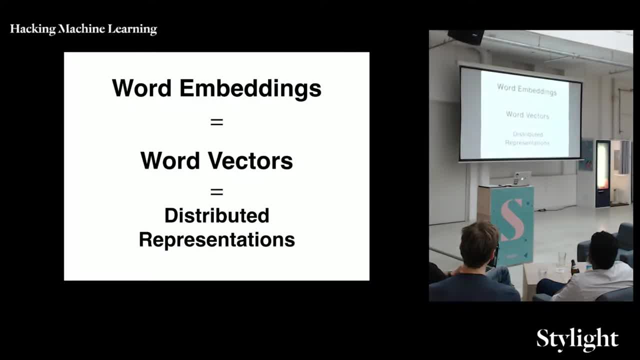 And then a bit of Python at the end. So terminology: word embeddings are vectors that represent words. So what you see here, they're all synonyms: word embeddings, word vectors, also semantic vectors, because, Okay, Okay. 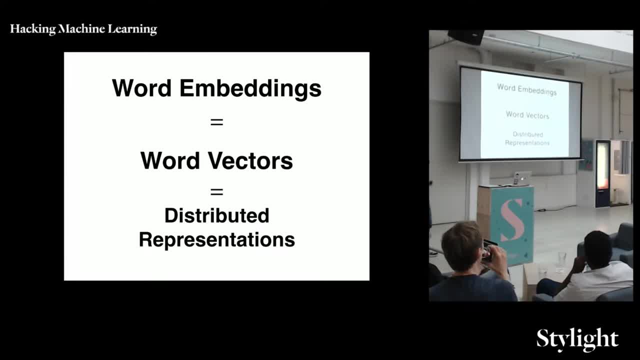 Okay. vectors capture the semantics of words And also distributed representations is another way to call word embeddings, because the meaning of a word is distributed across many dimensions. So why is this important? Well, in data mining, the way you represent your data is. 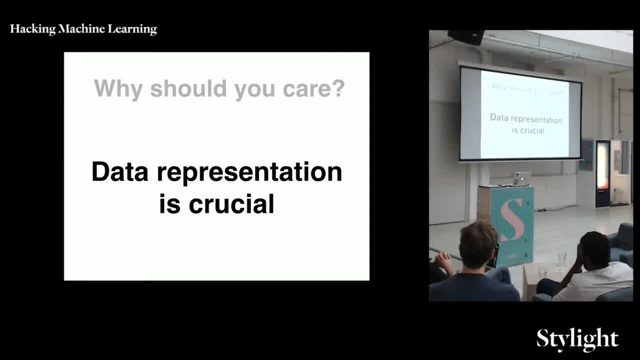 crucial for the success of your application, And in text mining that's the same story. So word embeddings are really interesting ways of representing text In terms of applications. where are these word embeddings useful? really? anything about text analytics is fair ground to try out some word embeddings. 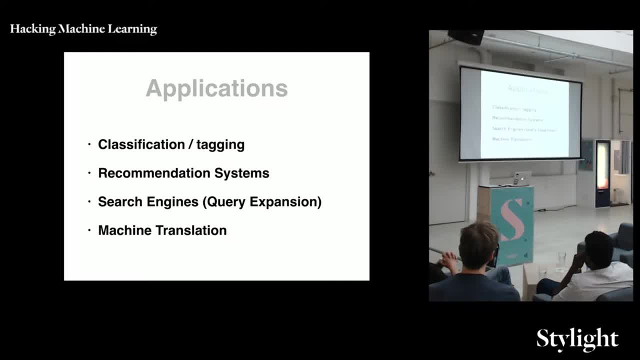 I'm just mentioning a few bullet points here, but that's not an exhaustive list. So classification or tagging, assigning classes to documents, recommendation systems, search engine, So you type in your query and then the search engine can expand your query and understand the 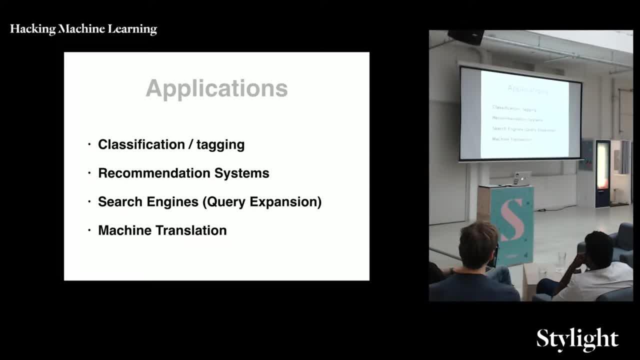 what you're trying to search, And then a bit more difficult machine translation, So going from English to any other language. These are all applications where word embeddings have been applied successfully, And there are many more. So really everything about text analytics is a fair game. 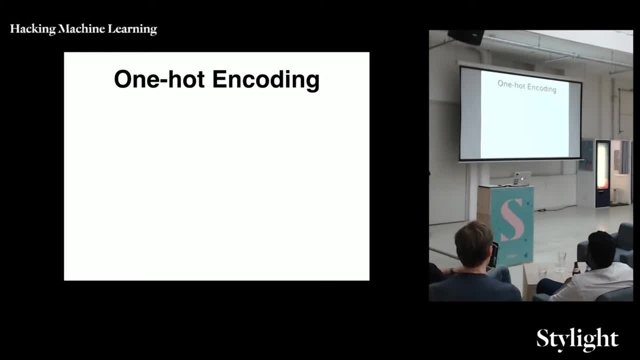 I want to start with a couple of ways of representing text. So the first one is the classic one-hot encoding. So in one-hot encoding you are going to have a lot of text, And in one-hot encoding you have lots of vectors. 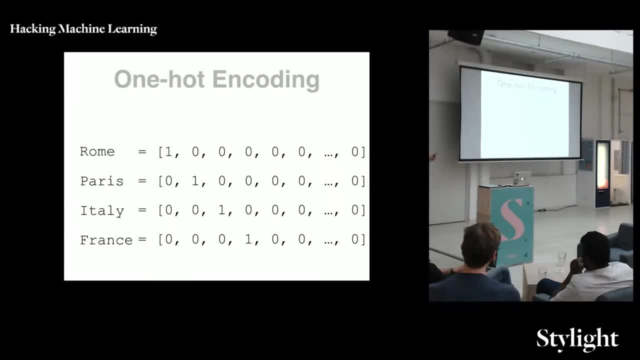 representing words And you see you have zeros everywhere And then you have only one bit being hot at a time. This is good to represent categorical data And you can use it to represent words as well. So essentially every dimension that you have there is. 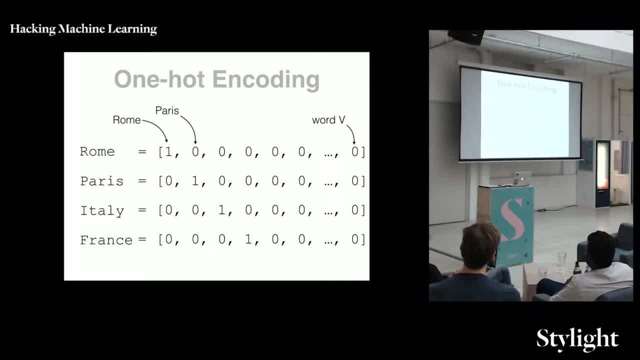 representing a word. So first bit for Rome, second bit for Paris, and so on until the last word. There's a problem here. We are basically Having a lot of dimensions, So the size of your vocabulary potentially is huge. 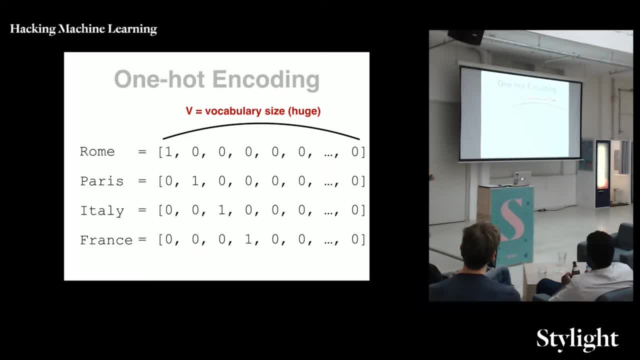 So there's a dimensionality problem And also we don't have any notion of similarity between these vectors, because these vectors don't have any dimension in common, So you cannot calculate easily any kind of similarity. Another approach to represent text is the. 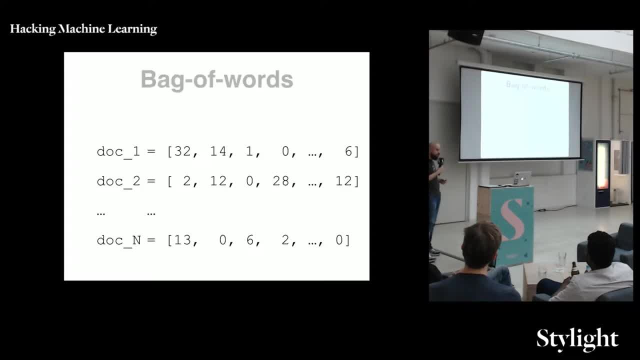 popular bag of words. This is used usually To represent documents, So with documents you also have vectors, for example. And again, each dimension is essentially representing a single word. This could be how many times you see the word Paris in document one. 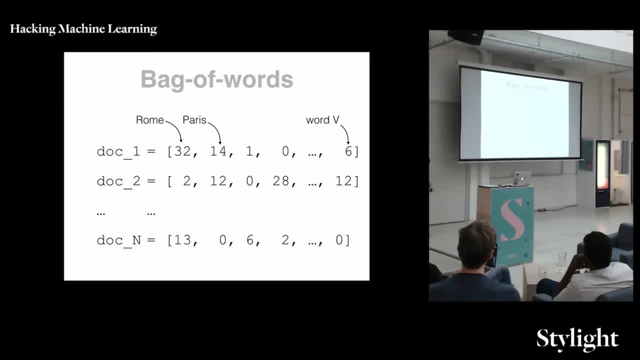 That's 14.. How many times you see the word Rome? That's 32.. That's a row count. You could normalize it in many other ways, But again you have a big number of dimensions And at least you start having some notion of similarity. 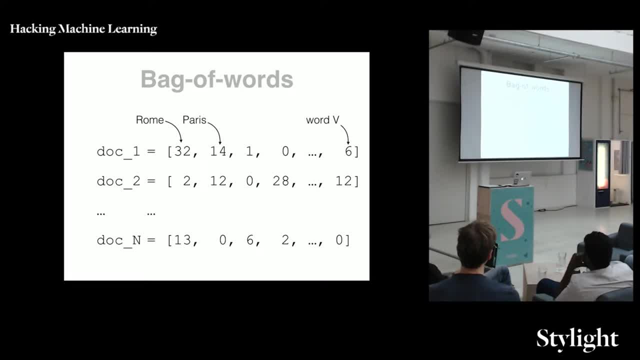 because you might have some dimensions in common here, So you can compute similarity between vectors. Now, moving on with word embeddings, So word embeddings are also vectors. The example is kind of made up just to showcase a couple of aspects of word embeddings. 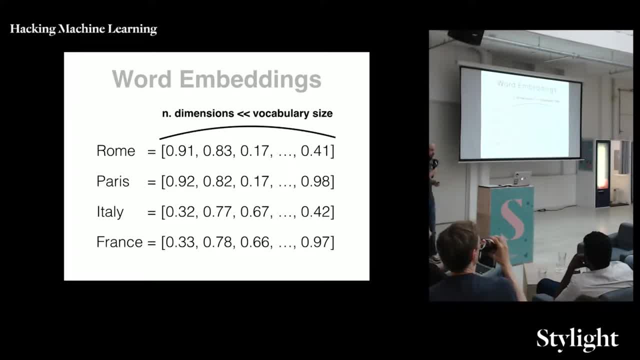 So what we want from word embeddings, we want the number of dimensions to be much, much smaller. So we want the number of dimensions to be much, much smaller, Smaller than the vocabulary size, And then we want to capture some ideas of similarity. 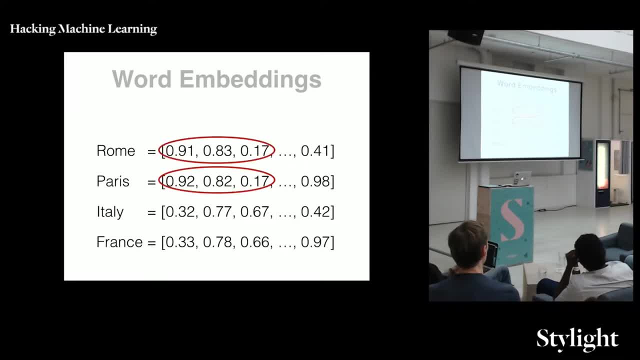 So, for example, Rome and Paris are somehow similar. They're both cities, They're both in Europe, They're both capitals, They are both nice places to visit. So a few dimensions. you see, the numbers are kind of close to each other. 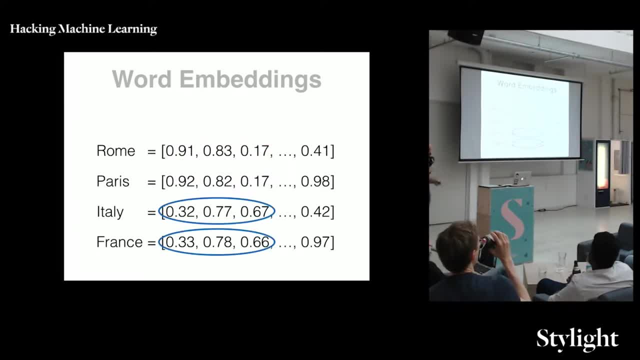 Similarly, Italy and France. they're both countries, They're both in Europe- Good wine, Good food And so on. So you want to capture this similarity with some dimensions. Also, Rome and Italy and Paris with France, they're kind of similar to each other in the sense. 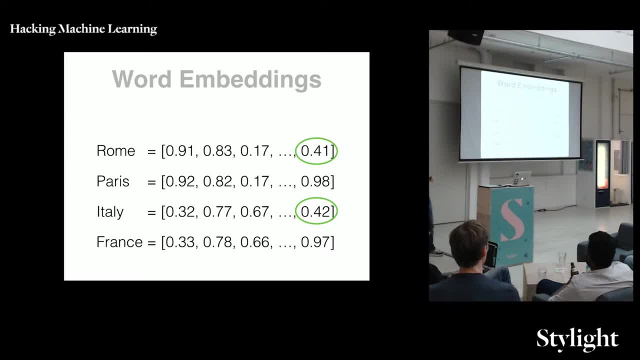 that there is a semantic relationship. So Rome is the capital of Italy and Paris is the capital of France. And this semantic relationship, you want it to be captured as well by some of the dimensions Once you go into pictures. if you try to picture it, you see. 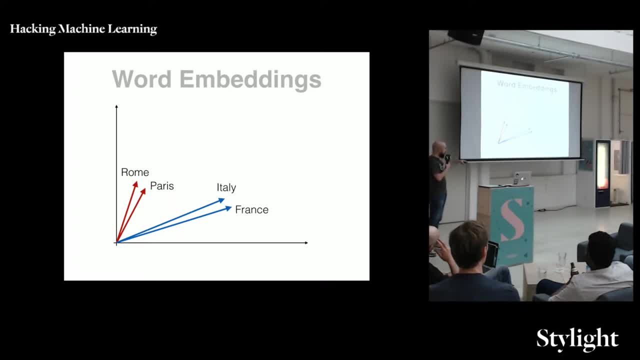 Rome and Paris as vectors. they're close to each other because they're similar. Italy and France as well, they're close to each other because they're similar. And you see, there's almost this direction, from Rome to Italy and from Paris to France, which is representing the relationship. 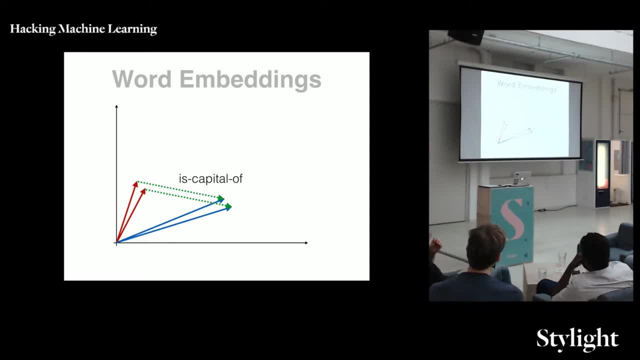 of being capital of, And that's the nice aspect- with word embeddings, So you can do vector arithmetics. You start with a vector for Paris, You add the vector for Italy And you remove the vector for France. You will end up with a vector which. 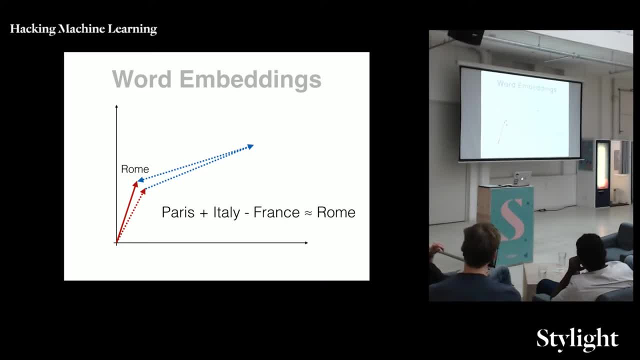 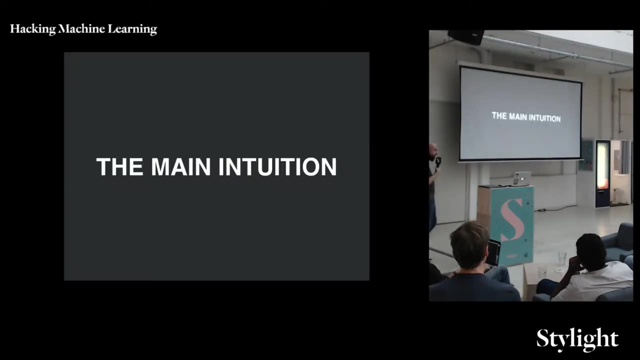 is very, very close to the vector for Rome, So you can perform this analogy task. And maybe you've seen before the king minus man, plus woman, equal queen. That's also an analogy. So we don't have vectors, yet We have language. 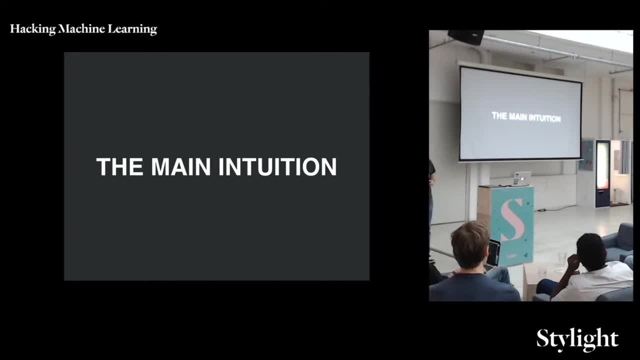 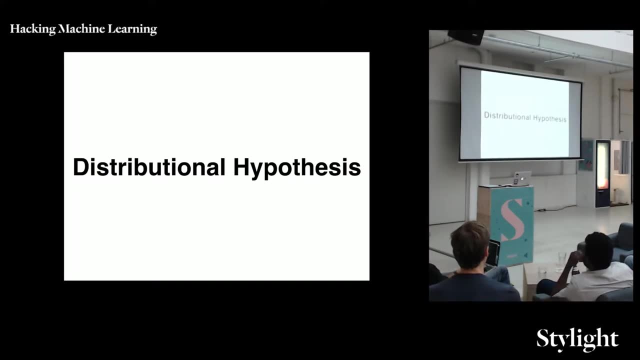 So what is the main linguistic intuition behind these models? That's called the language DISTRIBUTIONAL HYPOTHESIS, And this is nothing new. This goes back to the 50s And in particular you find the reference Usually every talk about word embedding. 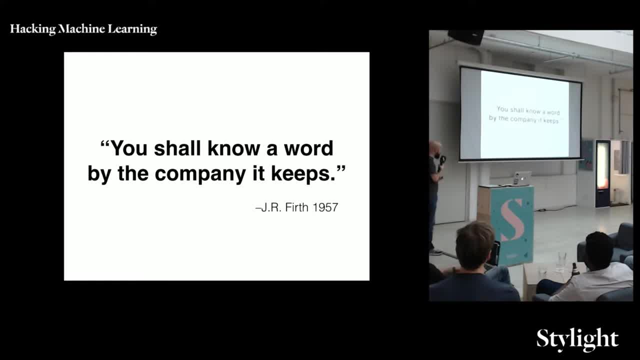 is a reference in this particular quote. You shall know a word by the company E-Keeps, by this British professor of linguistics, 1957.. And maybe it sounds a little bit too intellectual, So there is another one from a couple of years. 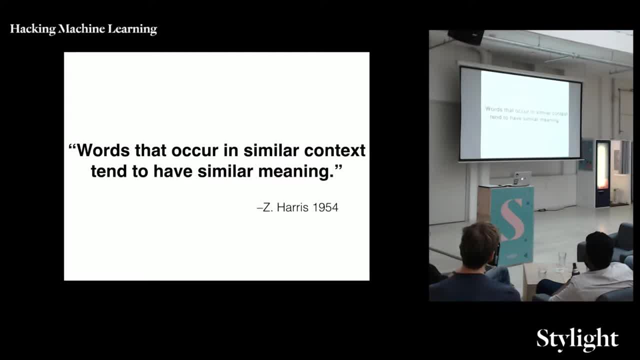 earlier, which is probably more clear. straightforward Words that occur in similar contexts tend to have similar meaning, So that's as simple as it is. We can use the context- so what's going on around a particular word- to approximate the meaning. 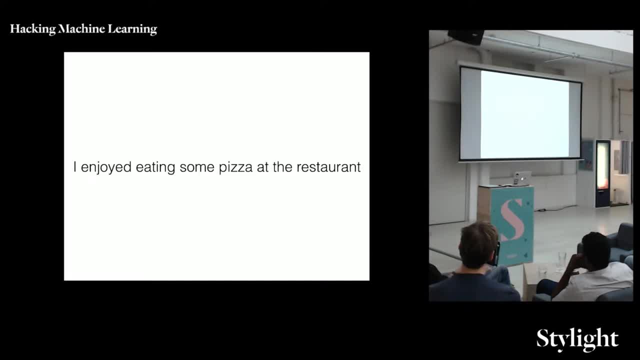 of the word itself And I want to give you an example. So this is a sentence. I enjoyed eating some pizza at the restaurant. We focus on what's important, So that's the focus word, the word pizza And everything else is the company E-Keeps. 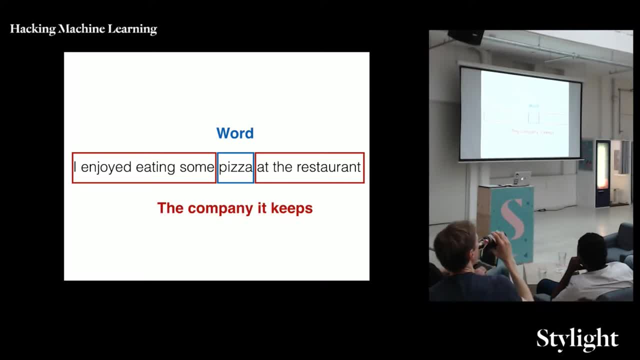 So that's the context of our word And essentially we can approximate the meaning of the word pizza just looking at the context. So pizza is something that we eat. Pizza is something that we have at the restaurant. Pizza is something that we enjoy. 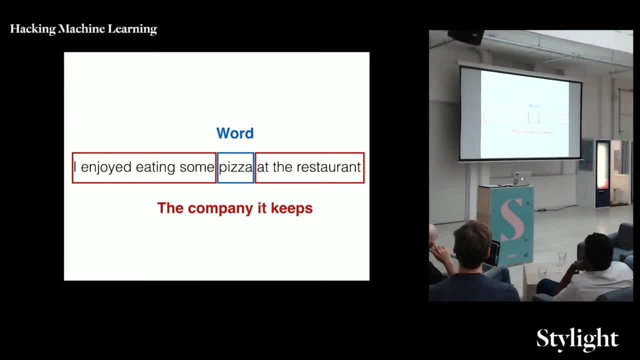 And then you scale it up on thousands of sentences. You see how the word pizza is used in the sentences And once you aggregate you end up with the true, deep meaning Of the word pizza. And now I give you a counter example. 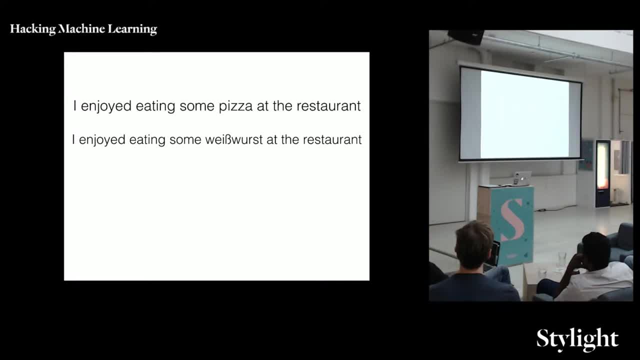 So you have two different sentences. I enjoyed eating some pizza at the restaurant And I enjoyed eating some Weisswurst. You just spell it right. Yeah, So these are two different focus words And maybe you already see where this is going. 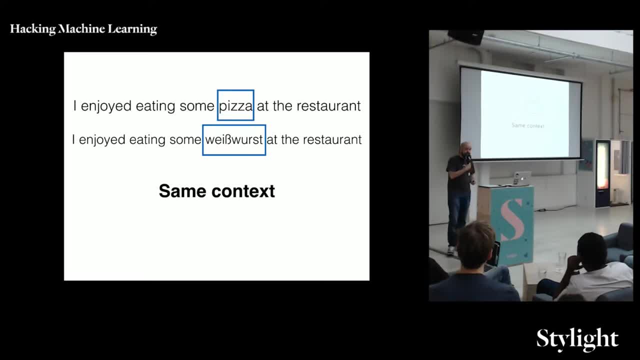 So we have the same context, According to what I told you so far. same context, same meaning. OK, So for some people, maybe having pizza or Weisswurst is the same thing. For me, this is kind of outrageous. Don't blame me. 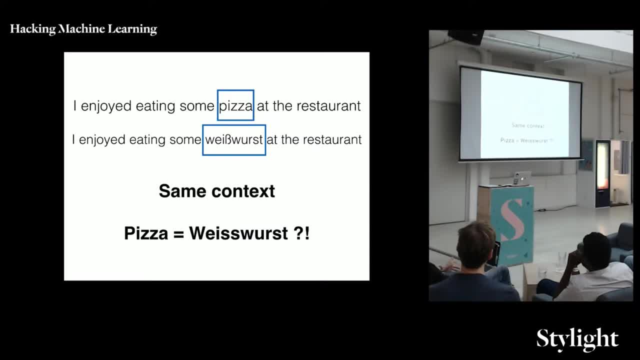 Blame the data. That's what the data look like. That's what the model is going to pick up. So this is just to have a bit of fun with a simple example, But really it opens for a discussion on data quality. 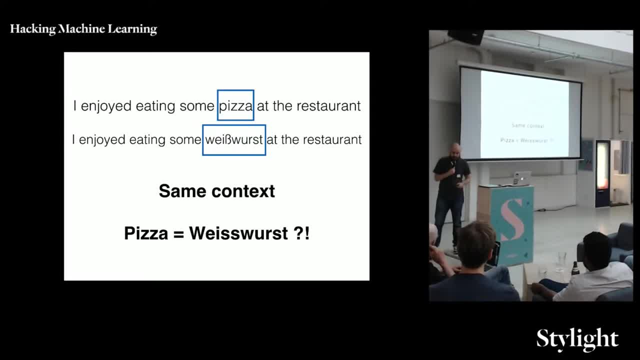 Your model is only going to be as good as your data, And possibly about ethics, because language is going to be biased. OK, It will pick up the biases from your culture And your model is going to pick up the biases from your language. 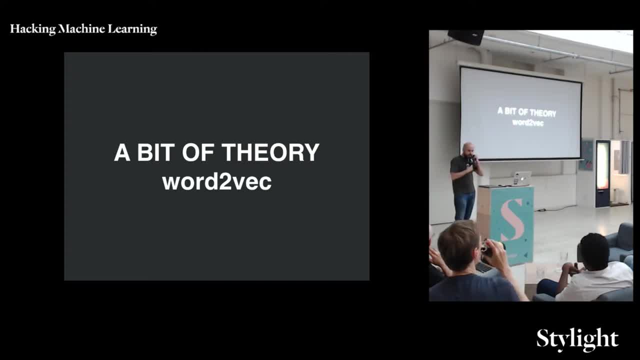 OK, Now, moving on with a bit of theory, I'm going to mention in particular the Word2Vec family of algorithms. So word embeddings are a family And Word2Vec is kind of a family within the family, And Word2Vec is what started all the interest a few years. 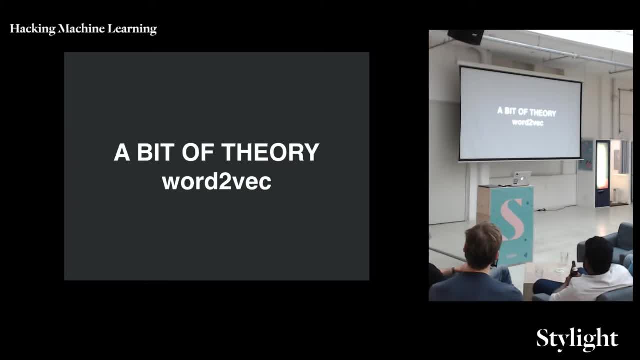 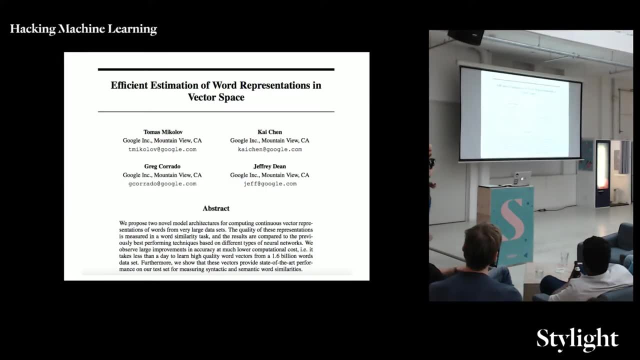 ago, around 2013,, on this word embeddings and on doing arithmetics with words. So this is work that has been done at Google. So Thomas Mikolov and colleagues published a couple of papers in 2013,. Efficient Estimation of Word Representations. 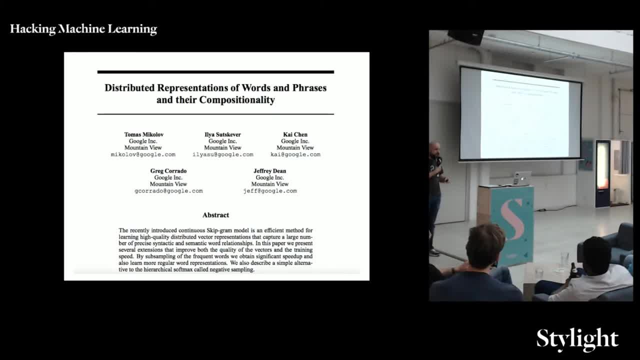 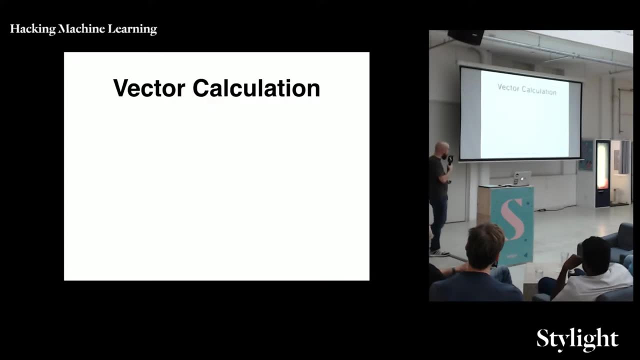 in Vector Space and also Distributed Representation of Word Phrases and Their Compositionality And the concepts from these papers. they ended up in what we know today as Word2Vec. So about the vector calculations? So how do we get vector from language? 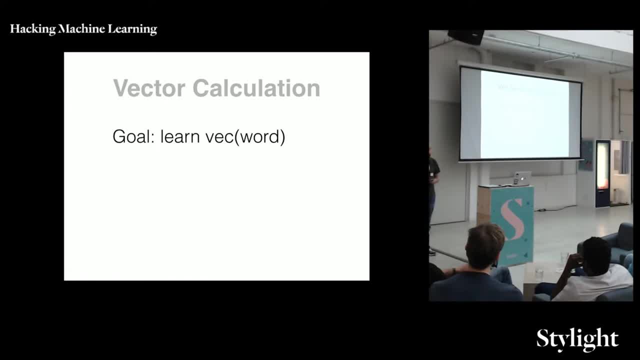 The goal, then, is learn vectors that represent words, And we're going to look at things from a distance, from the high level. So, first step, choose an objective function. Second step: initialize randomly our vectors And third step, Run stochastic gradient: descent until you. 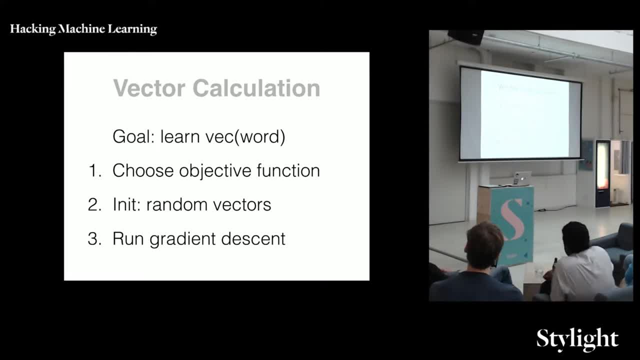 end up with the vectors, And if you've done some machine learning before, maybe you've seen the same approach applied to many other different contexts. So from a distance sometimes machine learning looks kind of everything the same. So what's interesting here is really 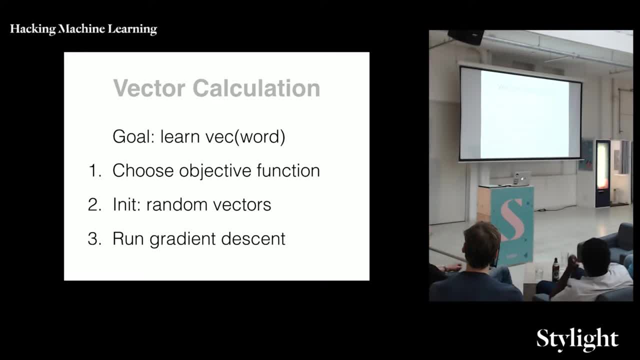 what's going on with the objective function? So the objective function is something that we want to maximize, And we call it the gain function, Or something that we want to minimize, And in that case we would call it a loss function. And I go back to the example. 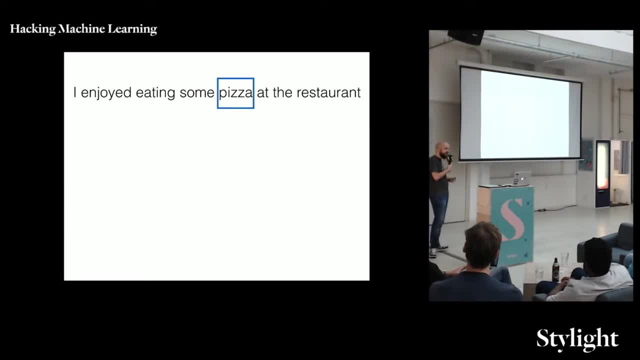 So we have the sentence, the focus word is pizza And that's our context. So the objective function in this case is we want to maximize the likelihood of observing the context given the focus word. In other words, we're going to end up. 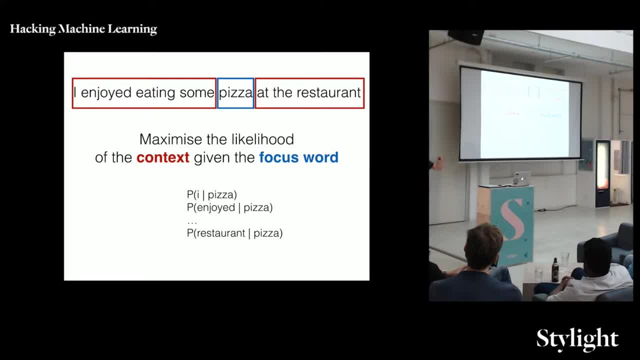 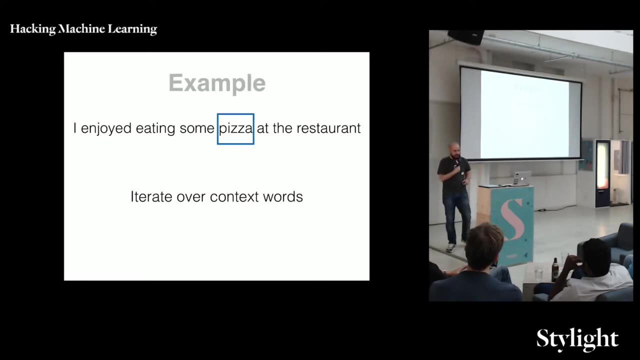 with a bunch of probabilities that look like this. So, probability of observing a context word given the focus word. Let me look at the example with a few more details. So we have our sentence as before, We have our focus word And we need to iterate over all the context words. 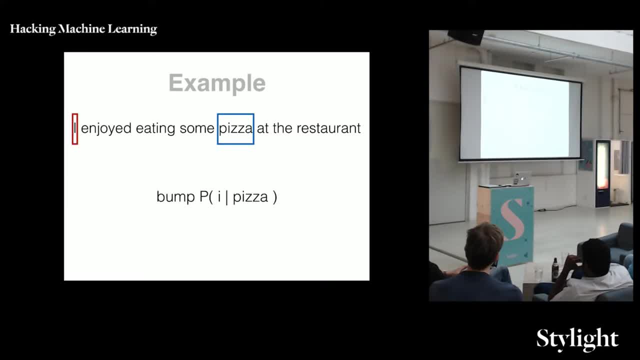 So we start from the beginning of the sentence. We see the word I, given that the focus word is pizza. So we bump up the probability of I Given pizza, And then we move on. We see the word enjoyed, Given pizza. 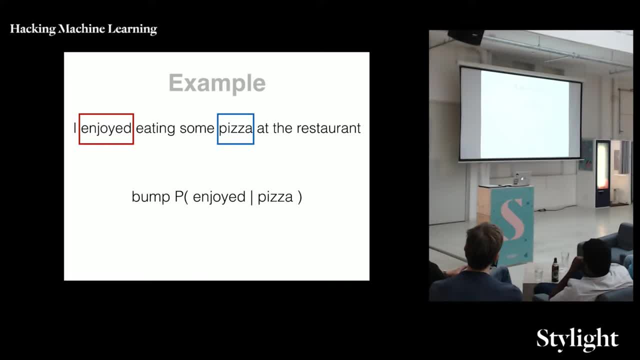 And we bump up the probability of enjoy given pizza. We see the word eating And we bump up the probability, And then again and again until the end of the sentence. Once we reach the end of the sentence, we move on to the next focus word. 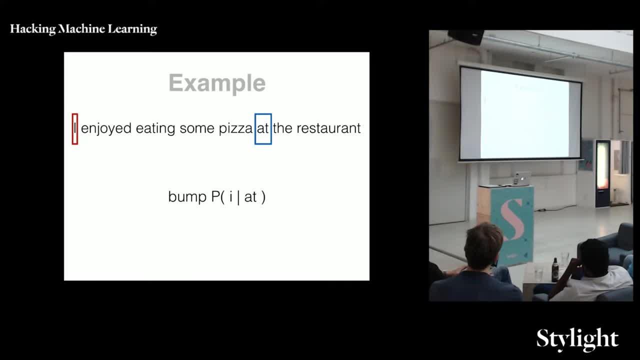 And we repeat the process. So, starting from the beginning, you see I given the word at Bump up the probability. You see, enjoyed Bump up the probability And then you see where this is going. So, essentially, two nested for loops. 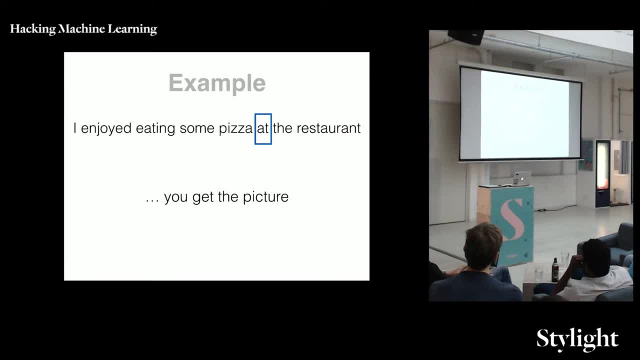 And then the core, the heart of the matter is bumping up these conditional probabilities. And I keep saying bump up the probabilities, but we haven't defined any probability yet. So what's the probability of eating pizza? Question mark: We can generalize. 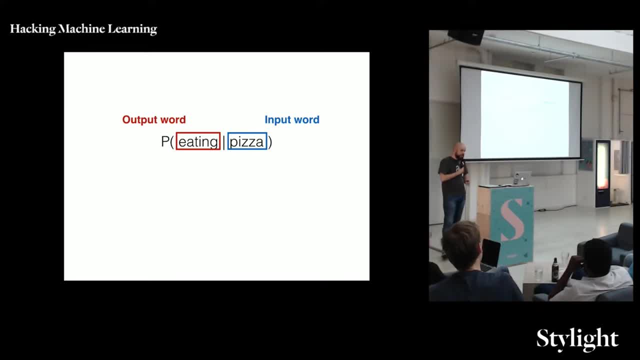 We call the condition, the word pizza, in this case the focus word, also input word, And we call the context word also output word, And we want these probabilities to be dependent on the vectors. So we kind of rephrase the probability. 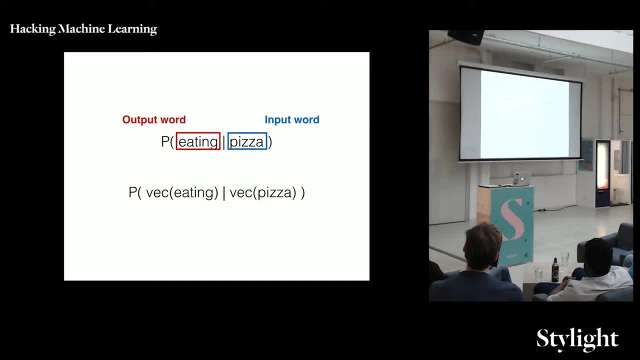 as probability between vectors. So, using this notion of input and output, we can rephrase it as observing or bumping up the probability of the output vector given the input vector. And again, we've been rephrasing but we haven't defined any probability yet. 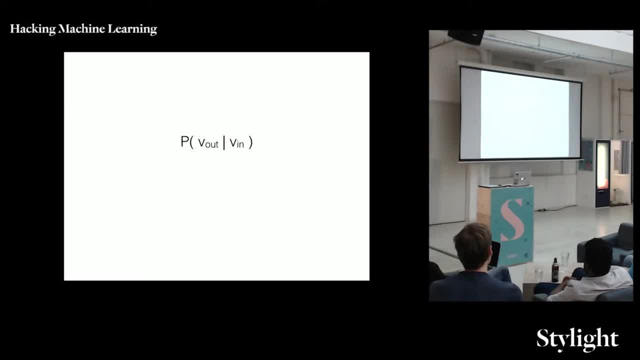 So we have this probability defined as vectors. Ideally we want the probability to be high if the vectors are similar. So first idea that comes to mind, use cosine similarity or other notions of vector similarity. That's a fair intuition. There's a problem here. 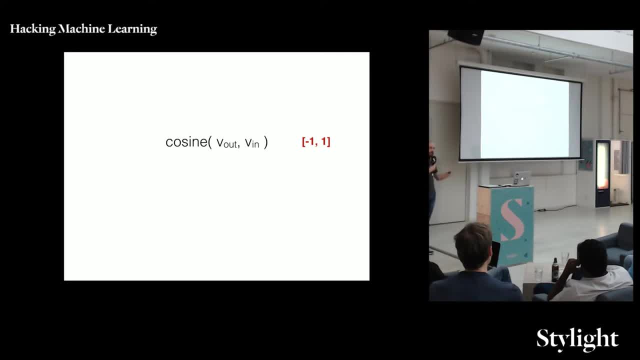 Cosine similarity is not a probability. It's a number between minus 1 and 1.. Next idea: take the cosine similarity and throw it into a softmax function. The softmax is used in many machine learning approaches. It gives you as output a number between 0 and 1.. 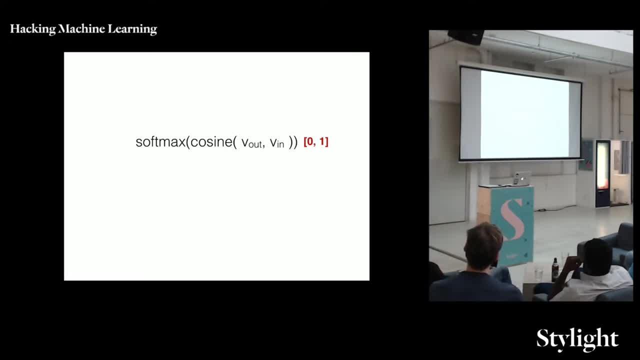 So it looks like a probability And it turns out it also has a probabilistic interpretation. If you want a formula, that's the formula. So the probability between vectors is essentially defined as the exponential of the cosine normalized over the sum across all the vocabulary. 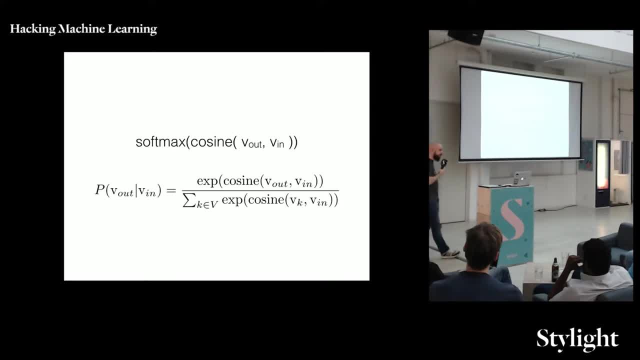 so all the exponentials for all the cosine similarities between output world and input world. If you have done some machine learning before, this is kind of maybe not new. If you're new to it, don't worry too much about the formula. Try to look at things from a distance. 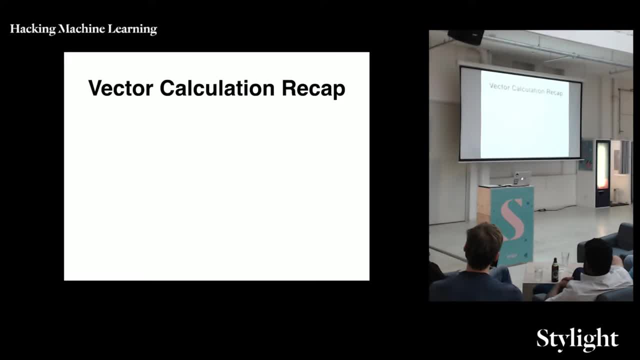 So just to recap this idea of computing vectors, what we've been doing, we've been learning word vectors using stochastic gradient descent on the softmax probability as defined before. So here you have all the ingredients that you need to apply this algorithm if you want to look it up. 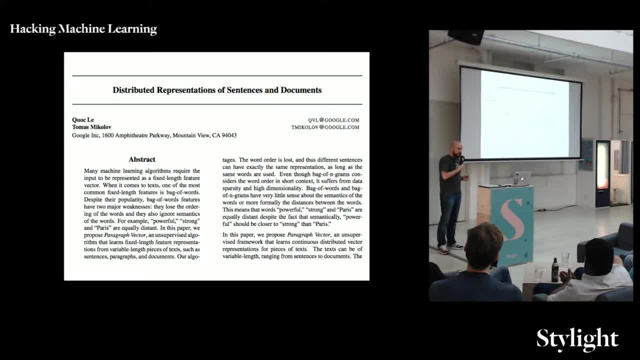 If the theory was not enough, there is more. It turned out. you can also learn not only vectors for representing sentences, but also for representing- sorry, not only for representing words, but also for representing sentences or documents. And that is a follow up work, also from Google. 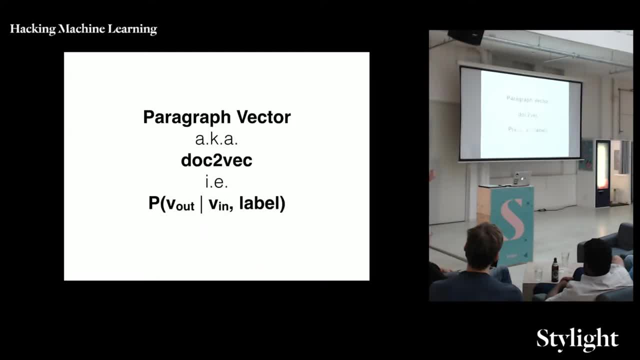 And in that paper they call this algorithm paragraph vector And, just as a reference to word2vec, they also call it doc2vec. And what we have here is pretty much the same. The only difference is how we define the probability between vectors. 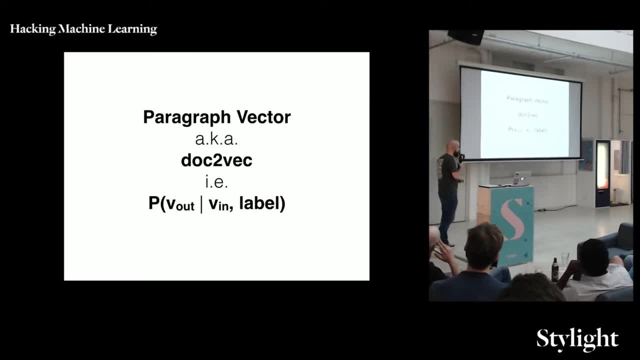 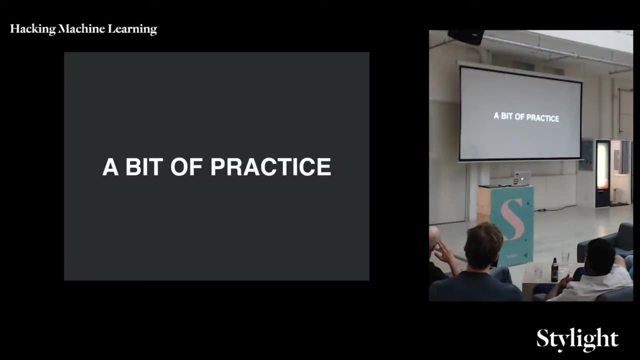 We also attach a label. It has a condition, And the label could be a sentence ID, a document ID, anything kind of ID that you use to group all your words into a particular paragraph. OK, and that's really enough for the theory. 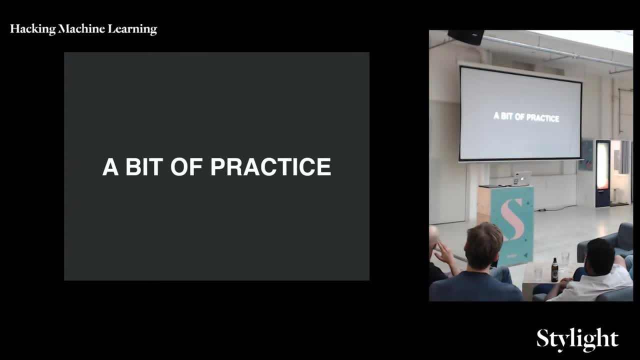 Of course I haven't given you too many details, but that's kind of the overall idea. Now moving on with the practice. So word2vec became popular because it was an academic success on one side and also because Google released the software as open source. 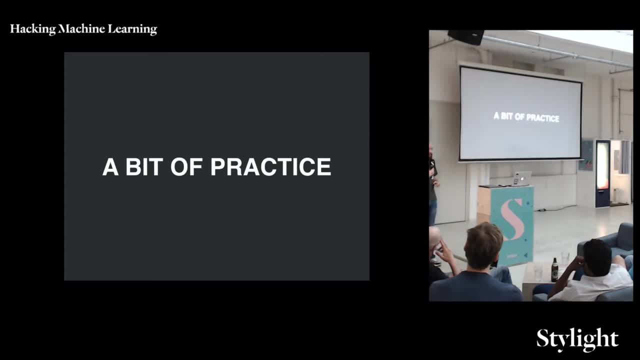 So there's a C library for training your vectors, And they also released the binary form for some vectors that were pre-trained on some Google News corpus- so billions of words that you can use. So essentially, you kill the training times to zero if you reuse those vectors. 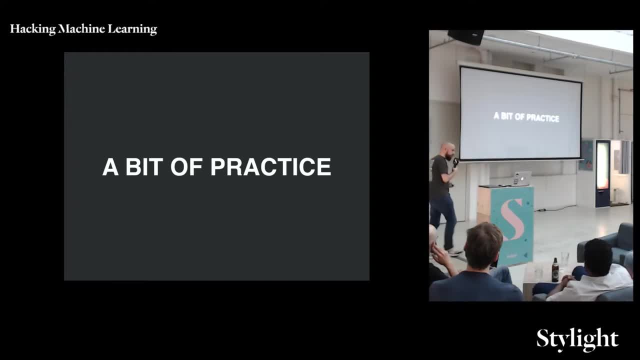 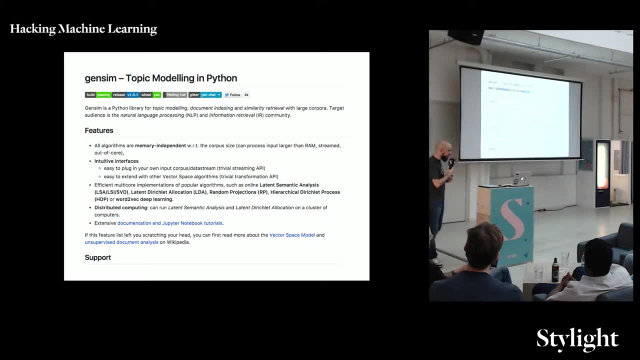 We're doing Python anyway, So let's look into Python. For Python, we have this library, Gensim. The pun line for them is topic modeling for humans. So what they do is they implement a bunch of NLP text analytics algorithms and they stick a nice interface. 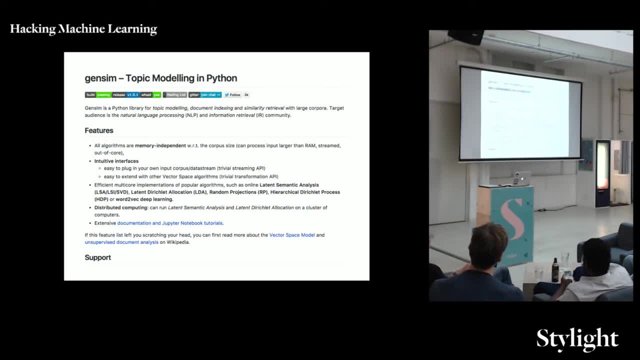 easy-to-use interface on top of it. And when they implemented the word2vec algorithms, it turned out the Gensim implementation in Python was faster than the original C implementation in Google, So that's how they got a lot of traction. 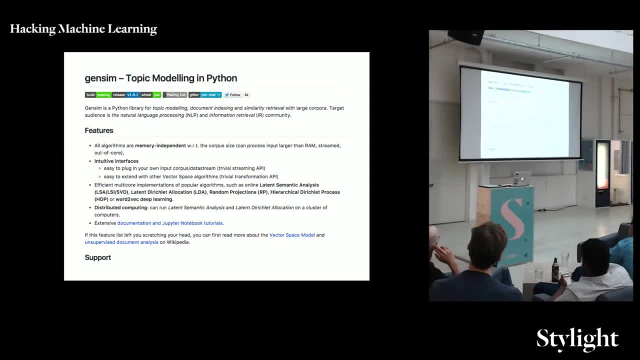 So Python faster than C. That's a lot of Cython and crazy NumPy kind of optimization, So that's how it was possible. Anyway, as users of the library, we only look at the interface, which is Python. So very, very simple, easy to use. 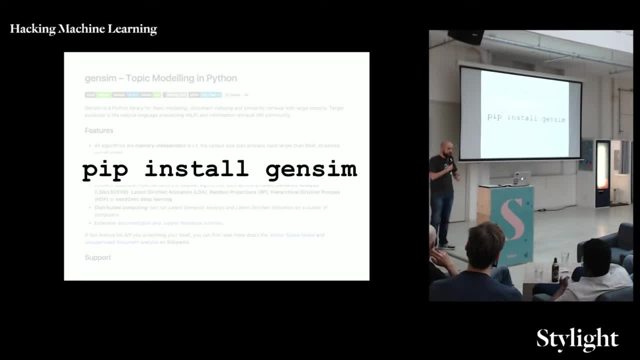 OK. So pip- install Gensim. Or, if you prefer, conda, Conda install Gensim. If you do data science, you should go with conda, And you're good to go, And I want to give you a couple of examples of how to use this vector. 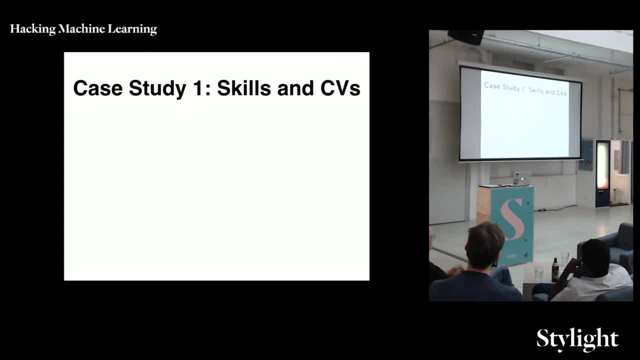 So this is some work that I did with a previous client of mine. They have a recruitment platform, So you upload your CV, Companies upload job specifications And then the machine learning magic in the middle tries to match the best people For the job. 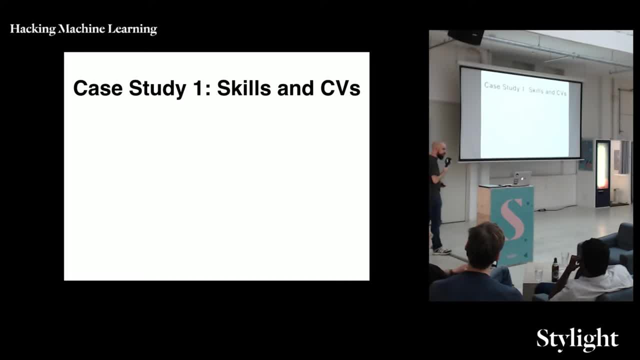 Essentially we were looking at CVs and the skills described in the CV. So we did a little bit of a pilot to see if word embeddings could be useful. We had a data set of 300,000 CVs. Each CV has a bunch of experiences. 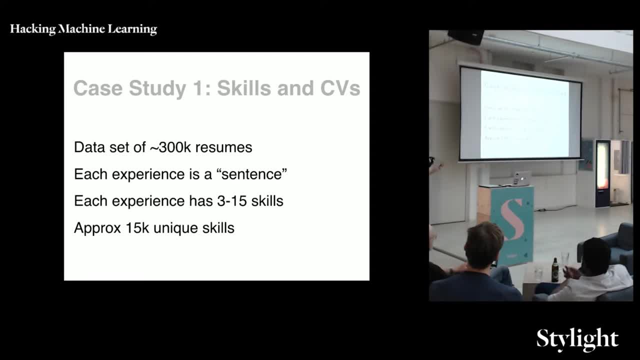 And we treat each experience as a sentence And each experience has a bunch of skills associated to it. Approximately, we had a vocabulary of 15,000.. 15,000 unique skills or unique words, So not a huge data set, And that's the Gensim part that you need. 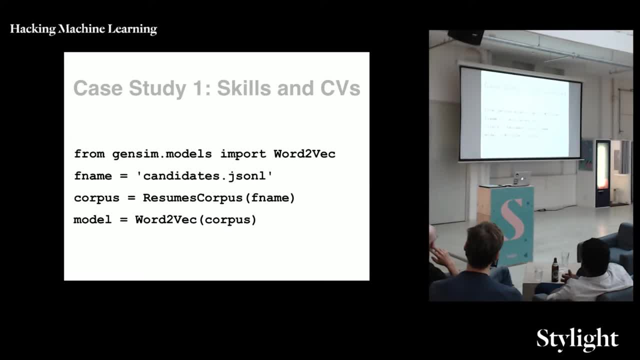 So essentially you import the class. You have your data set somewhere in JSON, CSV, any kind of format, It doesn't really matter. The custom part that you need to implement is your corpus reader. So the third line: the class will be probably a generator that yields. 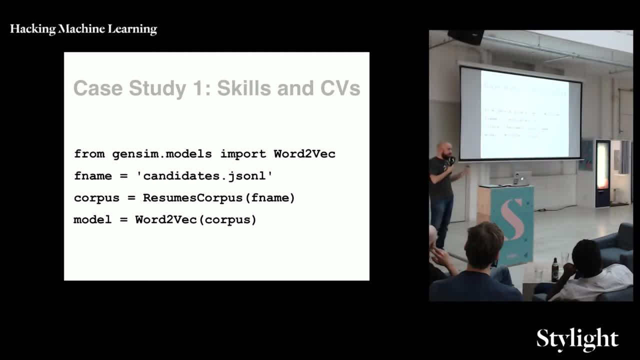 one experience at a time. OK, You don't need to load the whole data set in memory. Only one item, one sentence, one experience, in our case, at a time, And then you pass the generator to the Word2Vec class to load the model. 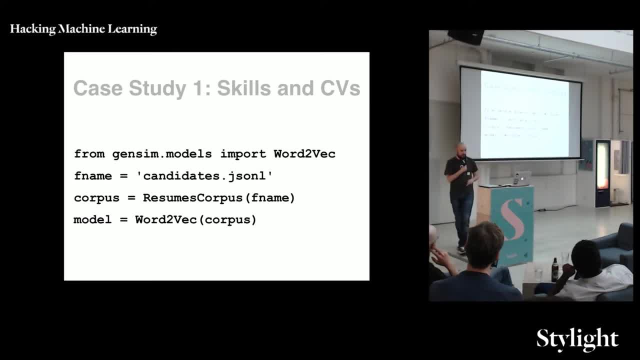 And there are a few extra arguments there that I'm kind of hiding the details. to keep it simple, You can choose a couple of options. You can choose the number of dimensions for the vectors and so on, So you end up with a bunch of vectors. 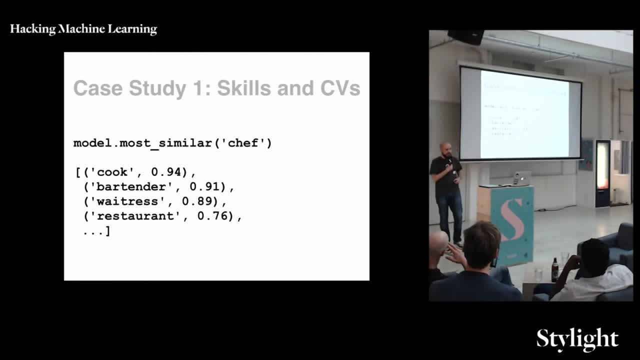 And you can look at vector similarities. So, for example, We have the word chef And we look at similar words And the first one is the most similar one to chef: cook. So they are synonyms. That's perfectly fine. And then, if you carry on, you see bartender, waitress restaurant. 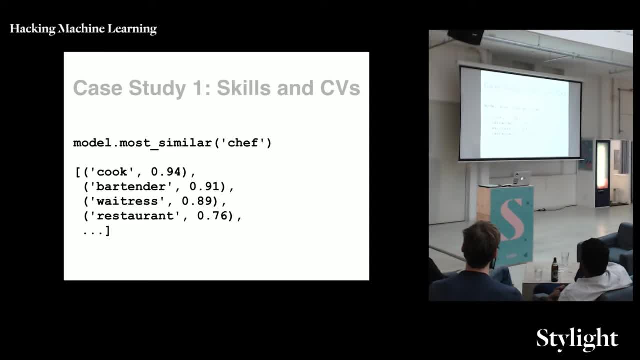 and other related words. These are not really synonyms But they are similar in the sense that they kind of belong together. OK, It's the restaurant business or the food industry, if you prefer. So it makes sense The word chef Also. you can use the word chef. 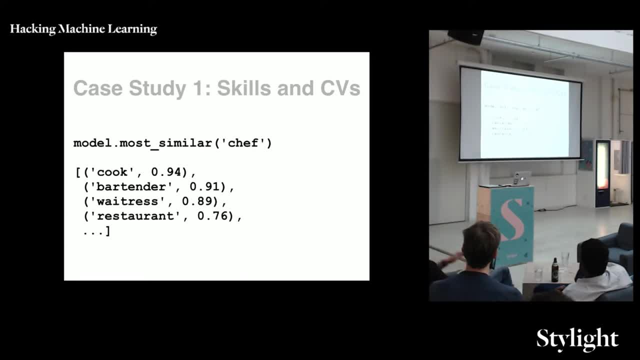 Chef also has another meaning. If you are an infrastructure engineer or devops, chef might be one of the tools that you use. It's the name of a library. So this is the magic: with word vectors You can do arithmetic. So take the vector for chef. 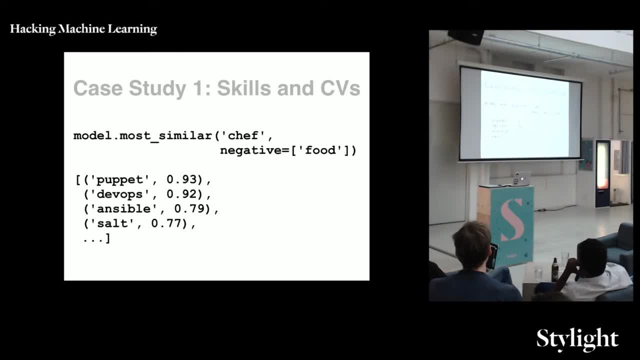 Remove the vector for food And you end up with a vector which is very, very similar to puppet ansible salt. These are all libraries in the devops kind of space, So essentially the model was able to pick up these nuances of the language. 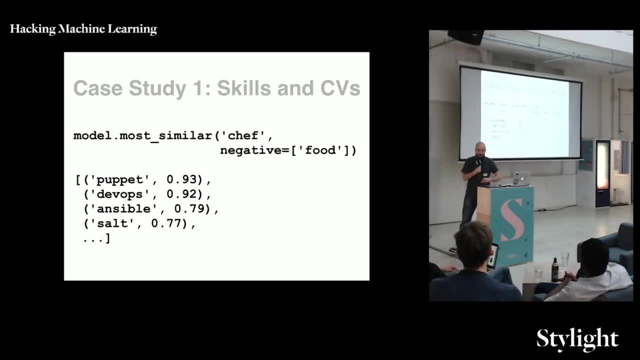 So the main meaning of the word chef is, let's say, the obvious one with the restaurant business, And then also doing this arithmetic, we were able to observe these kind of similarities. So the model was very, very useful for the data exploration. 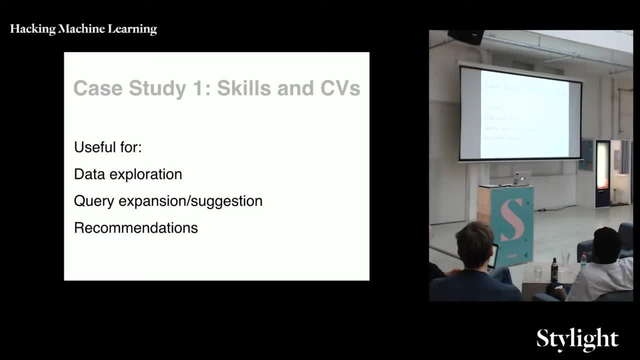 phase, really understanding our data. It was crucial And also we put it. We put it in production later for query expansion and query suggestions. So again, you type in your job spec as a company And you see what kind of skills belong together. 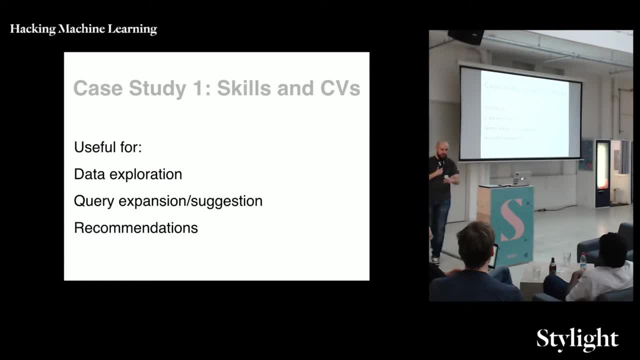 And finally for recommendations. so the algorithm for recommending people and jobs was influenced by the embeddings. Now, on a lighter note, different kind of use case, bit of a side project for me. I like data, I like Python, I like beer. 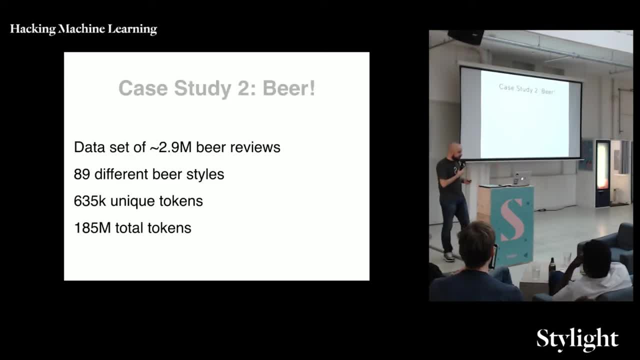 So why not putting everything together? So there's a data set for research of beer reviews- around 3 million documents- And all the beers are classified according to the beer style. So there are 89 different beer styles And you see the numbers. a bunch of and many, many words. 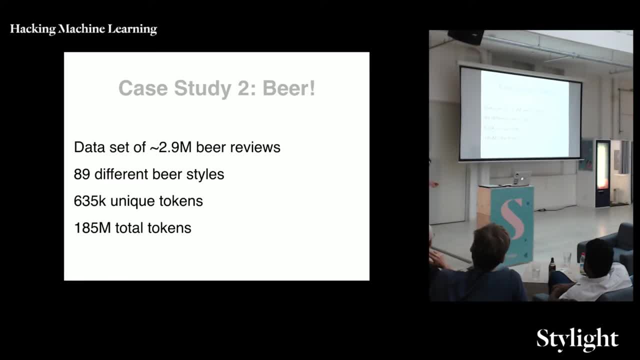 in total for this data set. I'm using Doc2Vac in this example, But the snippet looks very similar. So you import the class first, You have your data. This time it's CSV, Doesn't really matter. The third line: again, it will be your custom corpus reader. 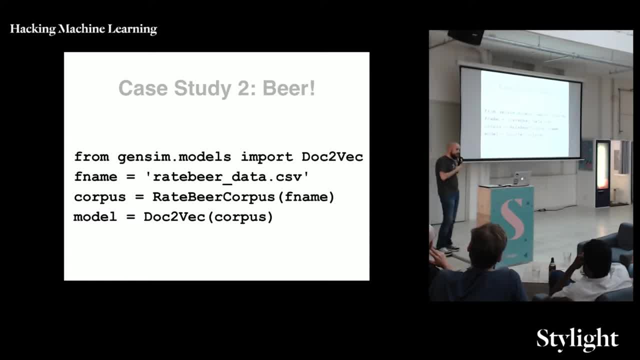 And because we are using Doc2Vac. in this case, the corpus reader is a generator that is going to yield one review together with the beer style as a label, If you remember the probability for Doc2Vac, it has an additional label And we use the. 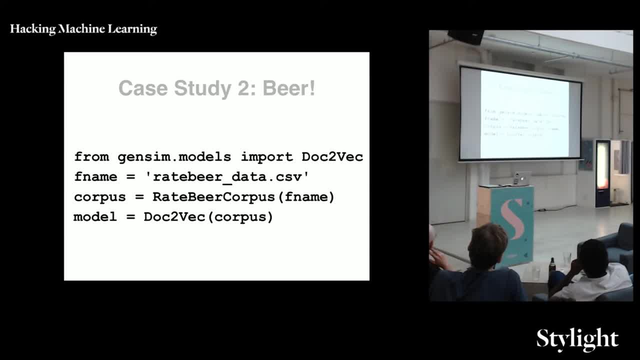 I use the beer style as a label, Load it as a model. About one gigabyte of data. so three million documents, one gigabyte of data, approximately 3.5 hours On my laptop. there's a bit of pre-processing. So the model maybe takes two and a half three hours. So suggestion is: remember to pickle. If you close your Jupyter notebook before pickling, you need to waste another 3.5 hours. So now you know that it took me seven hours the first time. 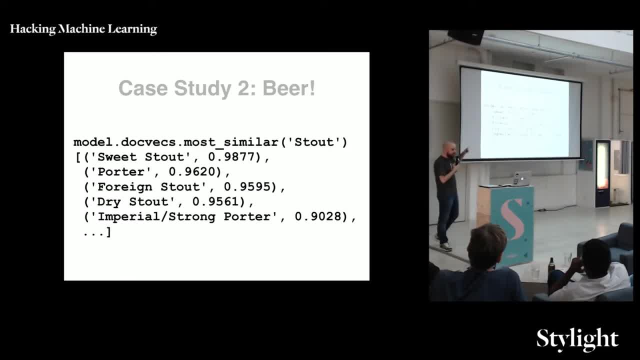 So we have document vectors here, so DocVacs, as you see, And we're looking for similarity between these labels, these beer styles. So stout is the name of a beer style, It's a type of dark beer And if you look at the most similar document IDs. 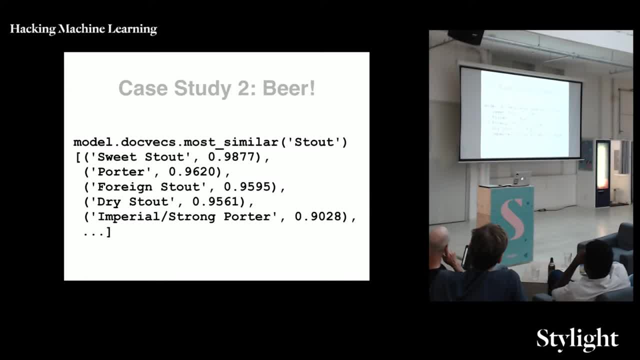 if you want, you see different variations of stout, so dry stout, sweet stout and so on. You see porter, which is also a dark English style of dark beer, And if you carry on with the list you will see all the sort of dunkel and still dark beers. 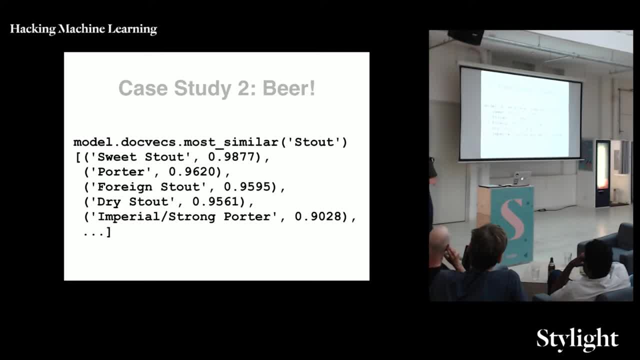 that are less similar to a stout, but still they belong to the darker sort of category. So it all makes sense. Once you load the Doc2Vac model, you also have vectors for words, So you still have the Word2Vac as well. 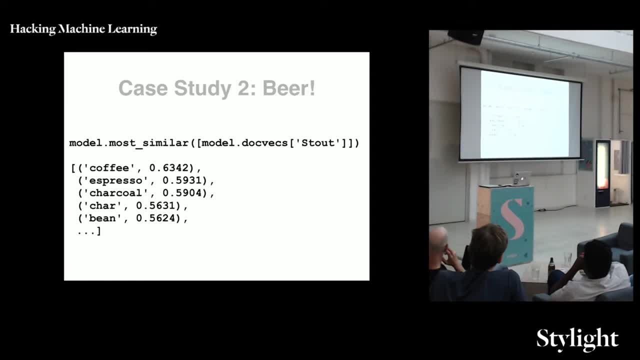 So you can check. OK, What are the most similar words used to represent the word stout. So stout is dark beer. The aroma should be kind of like coffee or chocolate, if you want. So you would find coffee and espresso as terms used to describe this kind of beer. 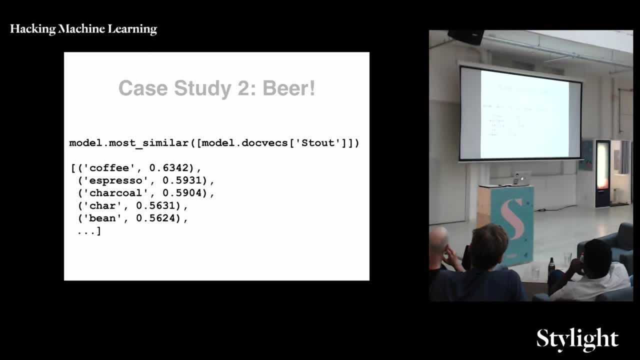 You see charcoal as well, because sometimes it's a little bit too much on the charcoal side. So that's also words that are used to describe the beer Bean. It's probably coffee bean as a phrase. It all makes sense, OK, if you know about beer. 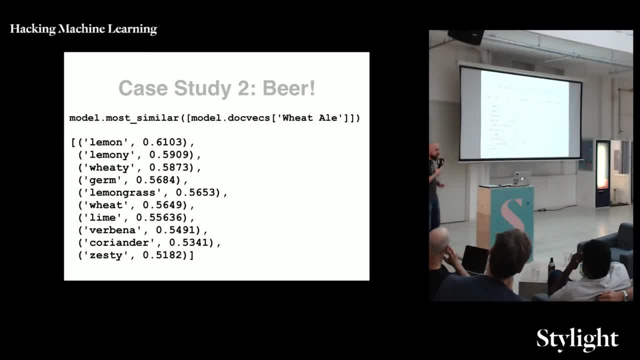 and about stout in particular. And as a counter example, let's say we look at wheat beer, wheat ale. The aroma is kind of like lemony, orangey zesty, So coriander seeds Again. it all makes sense. 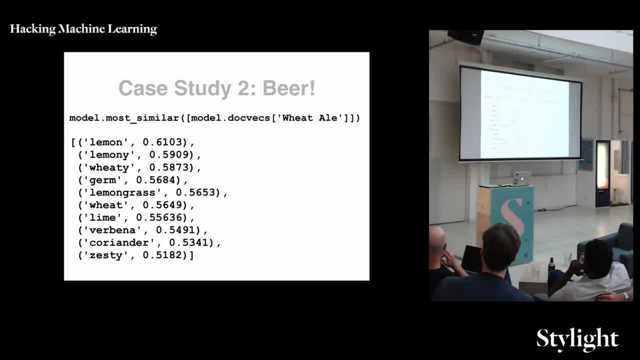 Wheat beer. so the data set is a bit biased in favor of American styles. So these are probably American wheat beer rather than Hefeweizen, if you want. So don't get too upset about this. That's just the data. 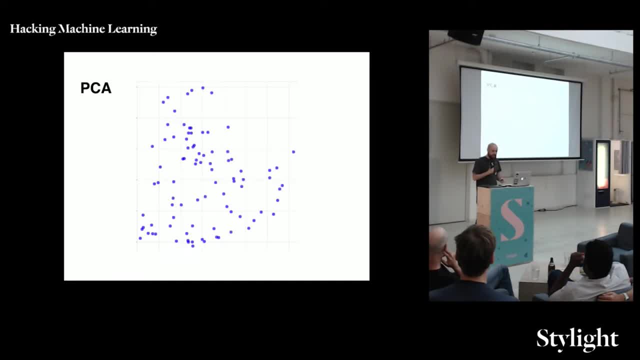 Now we have this: 89 different styles of beer. So I took the vectors. The vectors have a number of dimensions, 300, if I remember well. Throw them into principal component analysis, PCA to squeeze them into two vectors. so we could visualize. 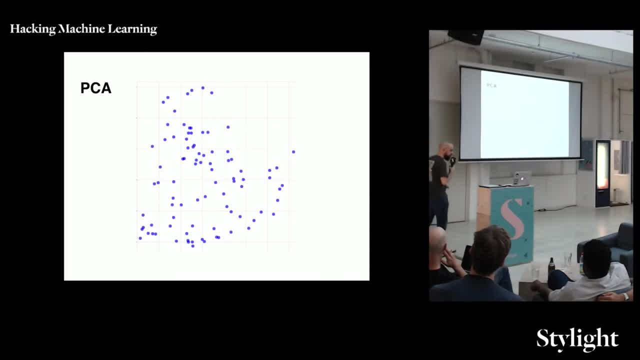 The vectors on the screen. We don't have a clear clustering here, but it still makes sense. So on one side we have all the dark beers, imperial stout, variations of stout, dunkel and whatnot. We have all these strong high-alcohol beers together. 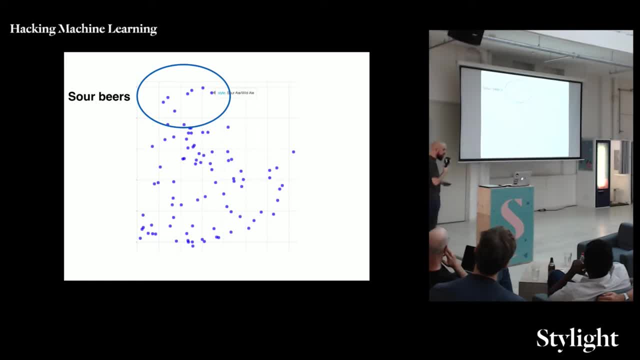 Then we have the sour beers. on a different league, Bottom left, we have all the lagers and peels, Kind of German and Eastern European styles, Wheat beer as well, and so on. So, even though you lose a lot of information when you go from 300 dimensions into two dimensions, 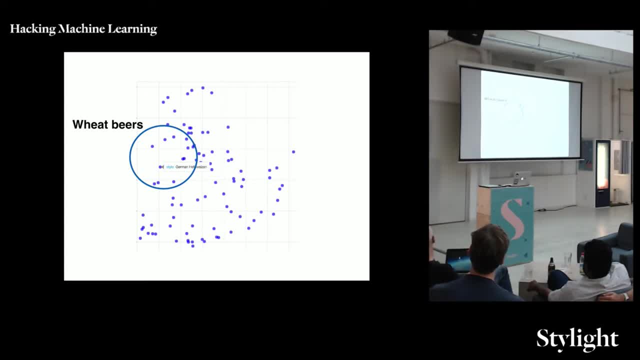 it still makes kind of sense And maybe completely random. but I noticed on the X dimension we have the color, So light beers are on the left and dark beers are on the right, and kind of brown, Orangy, copper kind of colors are in the middle. 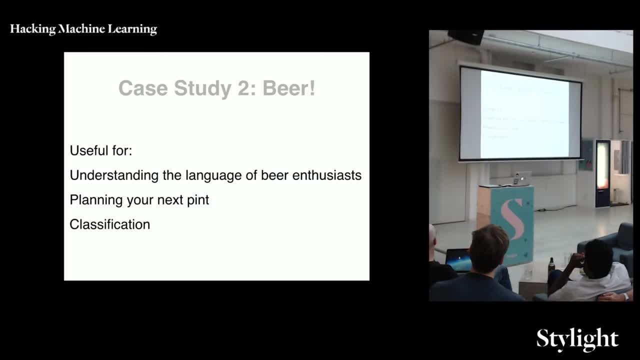 Maybe it's random, maybe it's not, So the obvious. How many connections did you reduce to those two? At the beginning? 300.. So each word vector has 300 dimensions. As a rule of thumb, not less than 100 and not more than 1,000.. 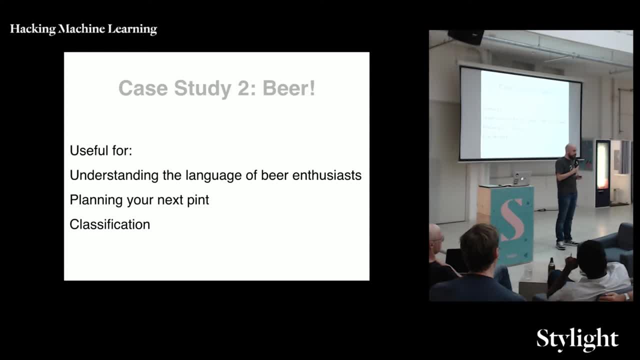 It's kind of a good starting point. So those are binary vectors. After PCA. you have two dimensions, yes, And the choice of two is just to plot it. You can do three and do a crazy bokeh. You know everything about it. 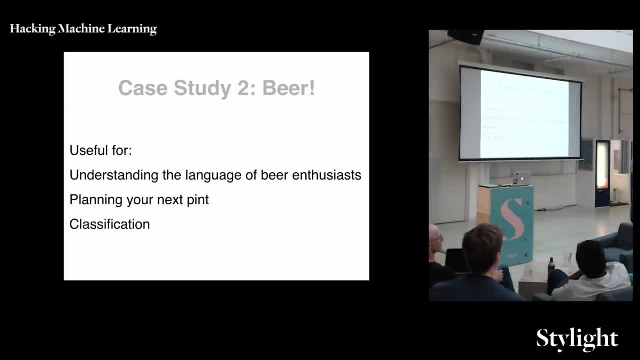 89 styles, 89 documents. Well, how many documents do you have? Three millions, Three million, Yes. And so how does that? How does that? Well, what's the complexity Like? would you scale it with n? squared or would you make more? 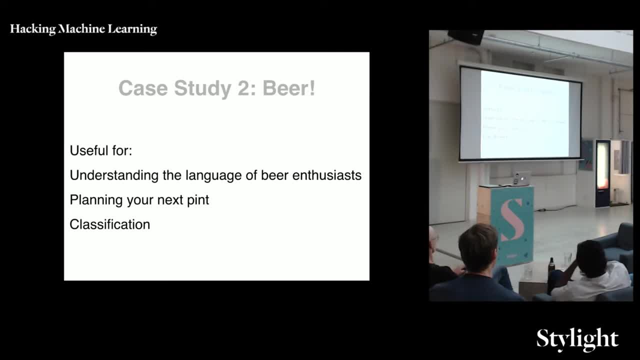 More on this later. It was a question about complexity and how it scales, So the obvious applications of this is kind of choosing my next beer, which is the point of this evening for me, right? Yeah, And just as a remark, It's really about understanding your data set. OK. 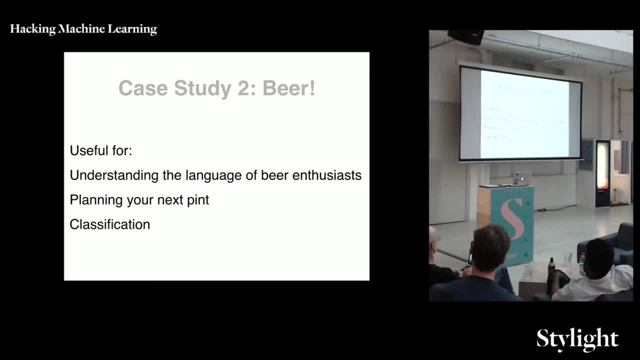 So this is about understanding the language, understanding the bias of the language and so on. It's really useful tool as exploratory analysis And also I apply it in classification. So comparing to a traditional bag-of-word approach, it was classifying better. 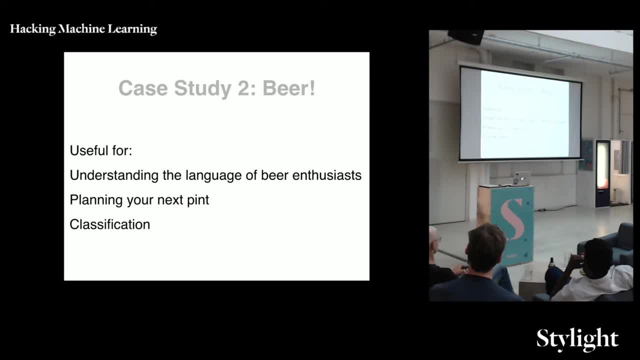 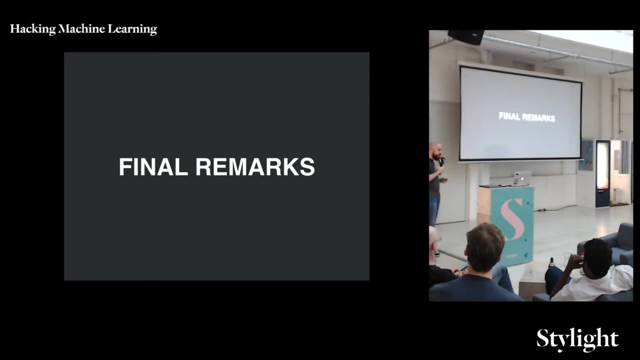 So, given a review, can you predict what's the beer style of this particular beer review? Using word embeddings gives you slightly better performances than that Traditional bag-of-words as kind of expected. OK, wrapping up, maybe you've seen this before. 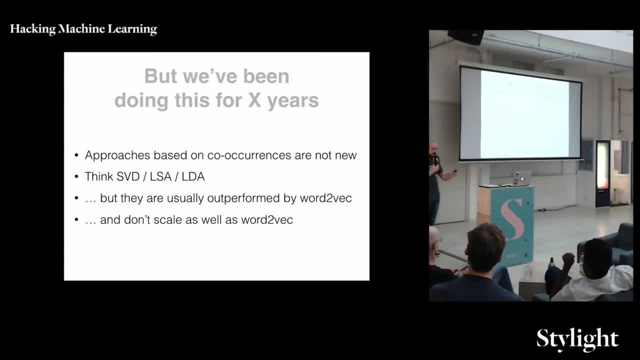 In particular, approaches in general based on co-occurrences of words that they've been around for a while: distributional hypothesis from the 50s and then LDA, LSA, singular value, decomposition and all the friends It's true. 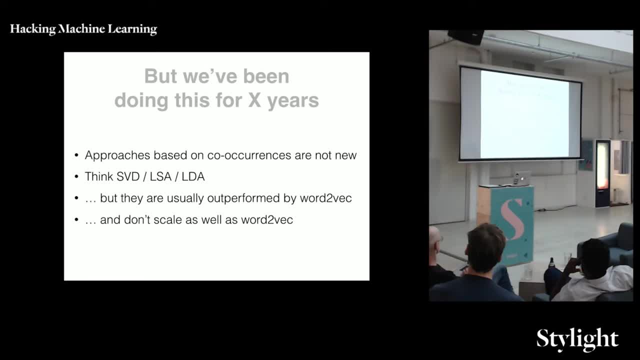 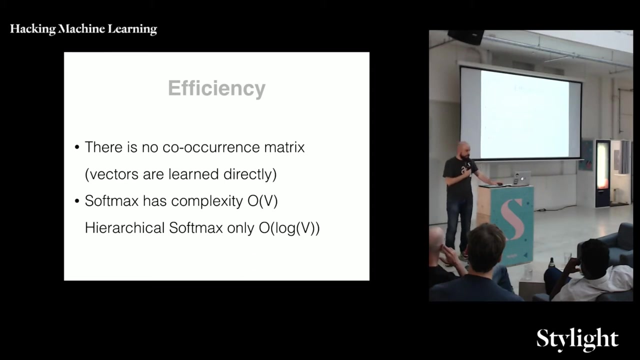 There's nothing new on this idea, but usually these approaches perform better than the word embeddings here, perform better than other traditional approaches And, in particular, they scale much better because of efficiency. They're based on co-occurrences, but there is no co-occurrence. 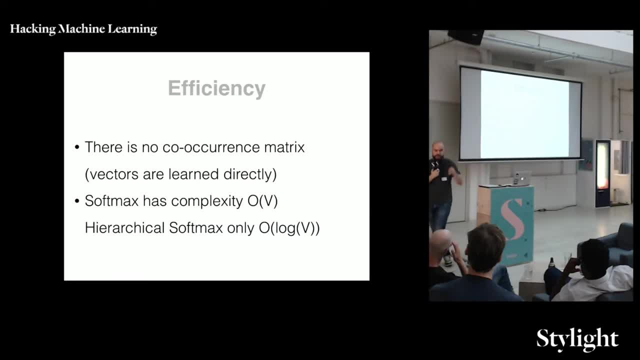 matrix in memory. You don't load the whole co-occurrence matrix in memory. You only learn the vectors directly In terms of complexity. so the softmax depends on you know it's normalized against the whole vocabulary. so linear complexity against the size of the vocabulary. 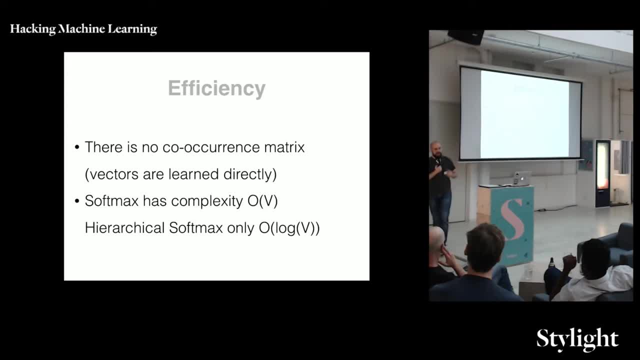 There's a trick for this, which is called hierarchical softmax, which is also described in one of those papers that I later referenced, And I don't remember all the details by heart. Essentially, there's a binary tree, There's a data structure, somewhere, so you go from linear. 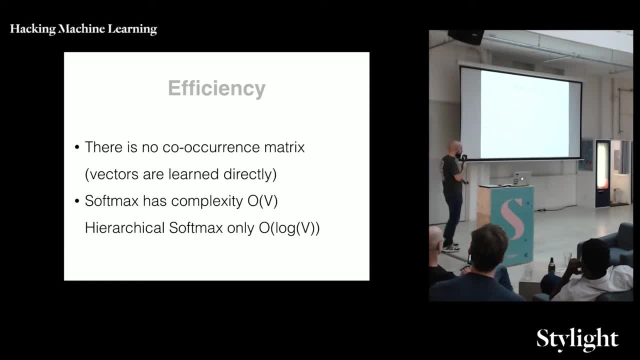 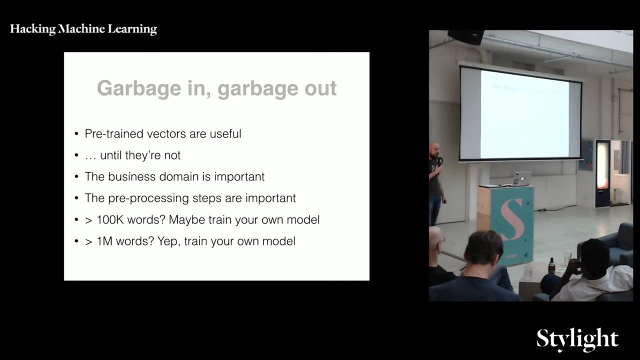 to log. It's proportional again to the size of the vocabulary Classic in machine learning: garbage in, garbage out. so the quality of your input will affect the quality of your output. So the pre-trained vectors that are given by Google for free, 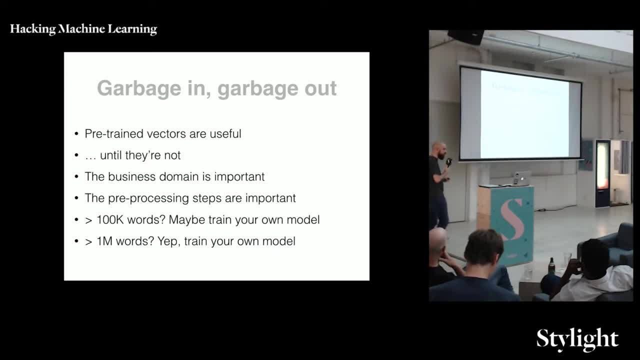 are useful until they're not useful anymore. In particular, the business domain is important, so they are pre-trained on Google News. So we're talking about specific kind of a you know language news and biased towards the US, so US-oriented kind of news. 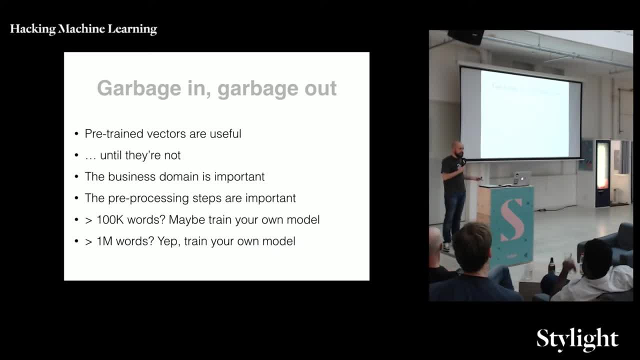 And the pre-processing steps are still important. so what you feed into the algorithm is still important. So the suggestion is: if you have enough data, train your own model. So, as a rule of thumb, 100,000 words, probably you can pick up some of the aspects of the language. 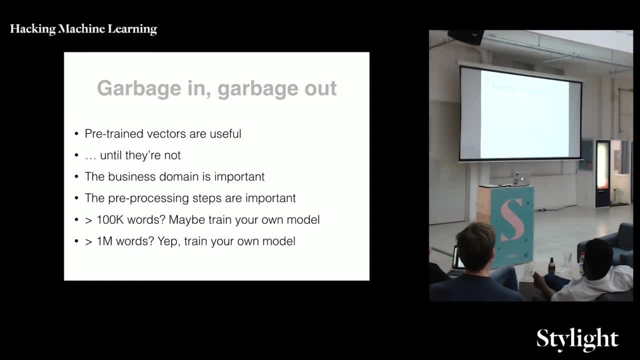 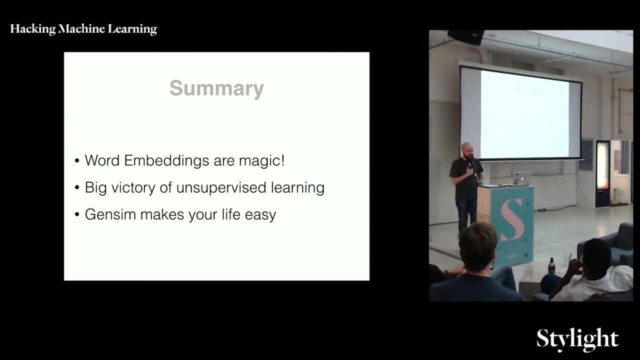 or maybe not. If you have more than one million words, definitely train your own model. That's not a big data set. OK, So that's a generic suggestion for this And just wrapping up: the first time you see these word embeddings and you do arithmetics, it looks like magic. 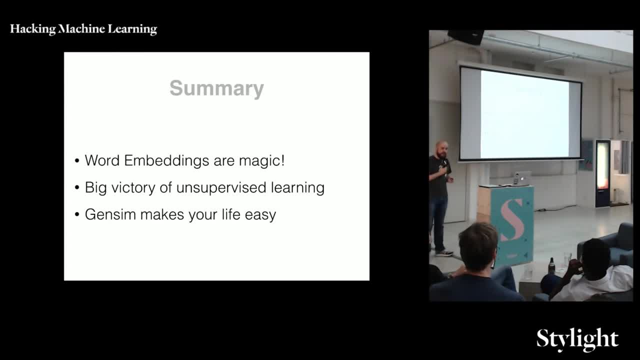 It's really just a smart application of unsupervised learning, And if you don't care about the theory, I don't blame you. You can just use Python, a few lines of Gensim and your life is easy. I just want to reference a couple of things. 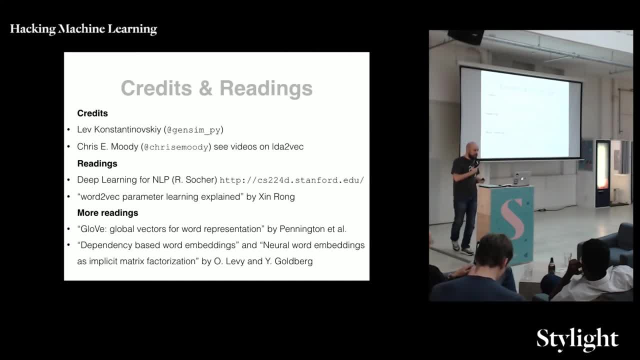 thank a couple of people. So Lev is one of the maintainer of Gensim. He's a friend of mine also. He's traveling around the world, so sometimes he's in London And we've been talking a lot about word embeddings. 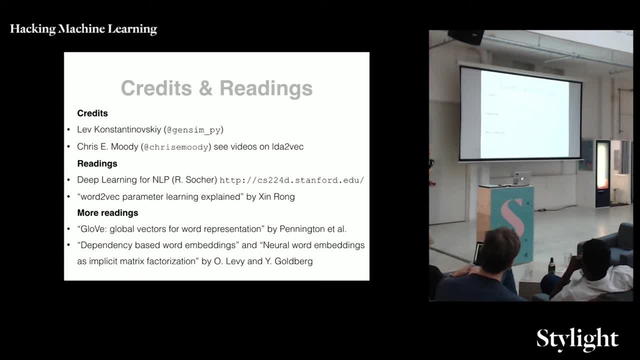 and the work they've been doing on Gensim. And Chris Moody- this guy I never met, I've just seen a few of his videos. He has a very nice explanation of word embeddings And he's a great guy. And he has also this joint LDA and word embedding model. 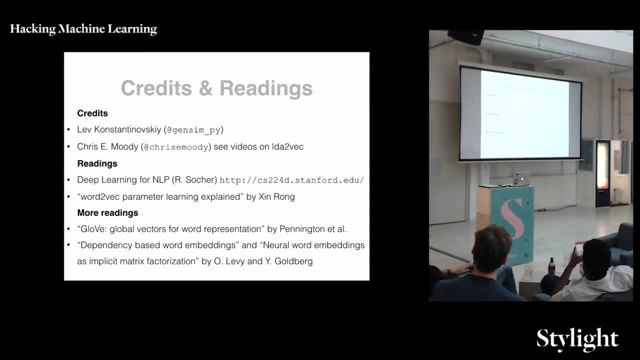 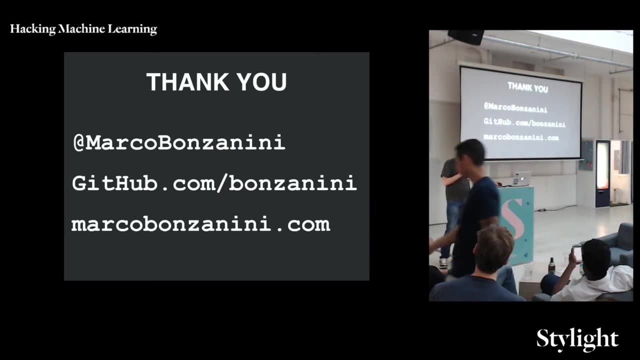 that he calls LDA2Vec And, if you want to know more, the usual suspect Stanford and a lot of material online for the Word2Vec. OK, that's essentially closing the talk for me. I believe we have a few minutes for questions. 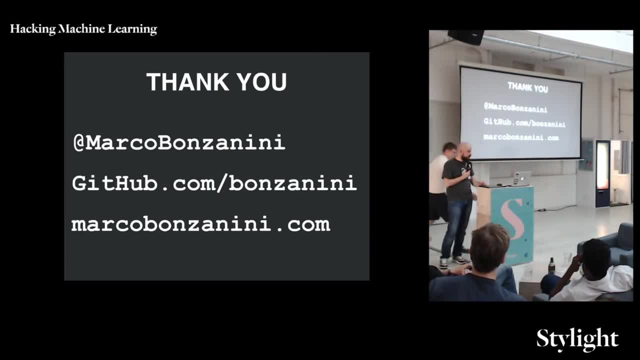 I'll be around anyway And I'm easy to find online as well. Thank you, Nice time for questions. Can you give examples for the 300 dimensions And how do you define them really? Is that by the algorithm or is there some human interaction? 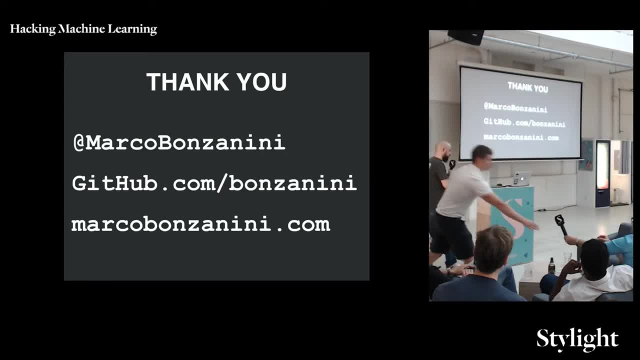 How I define the dimensions. Yes, So the idea is I don't want a huge number of dimensions, So the vectors have. it's easier to kind of handle this kind of problem. As a rule of thumb, as I mentioned earlier, less than 100 dimensions, maybe you. 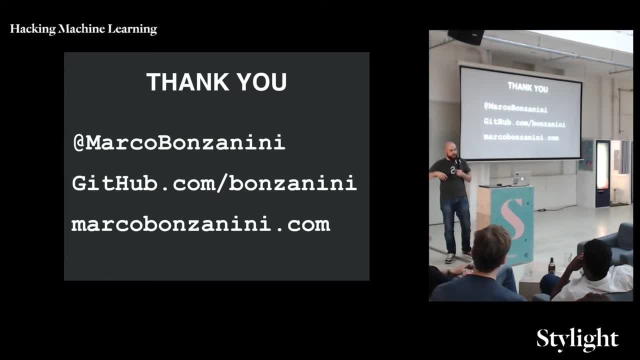 don't pick up these notions of similarities. And more than 1,000, it doesn't give you more. So people usually start with 200, 300 dimensions. That's an empirical kind of observation. That's what you see in many, many papers. 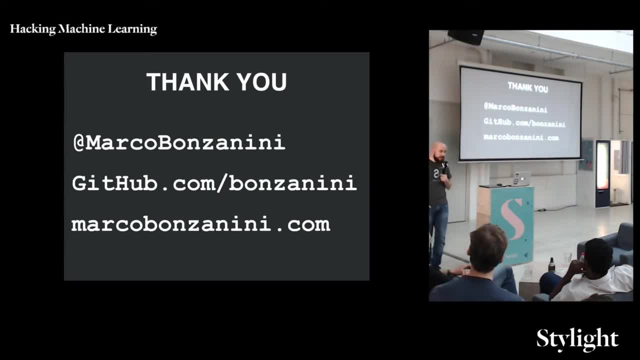 And this number is purely empirical. So you define. You can define how many dimensions you want. It's up to you. By default, if I remember well, you have 300.. When you pass the corpus to the word2vec class, 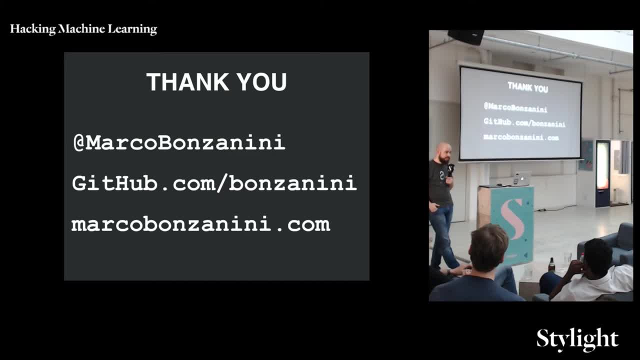 you can define how many dimensions you want. As simple as that. So you take the 300, the number of 300s and then you count the words and you take the top 300 words and those are No. You initialize the vectors randomly. 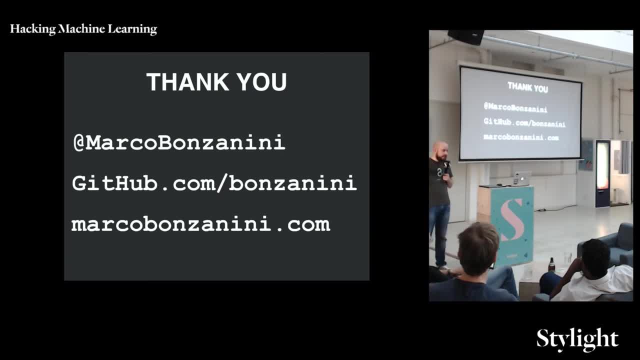 So you have 300 random numbers And then the algorithm looks at the co-occurrences and it will bump up using stochastic gradient descent. So stochastic gradient descent has the objective of maximizing the probability of the context world, given the focus world. So it's run by stochastic gradient descent. 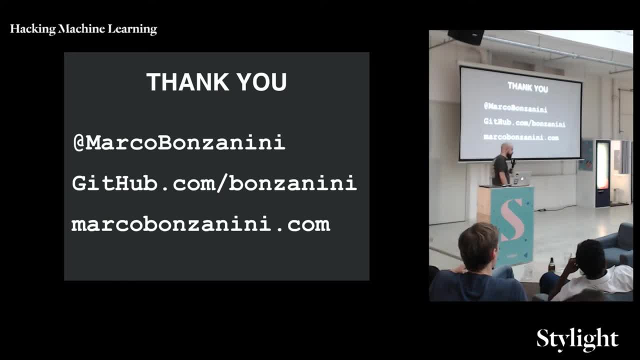 This is pretty cool. Thanks for sharing. This is pretty fun things. So I didn't understand. I didn't understand. I didn't understand the complexity only depending on vocabulary size. I have a vocabulary of 30,000 words, which is roughly the English language. 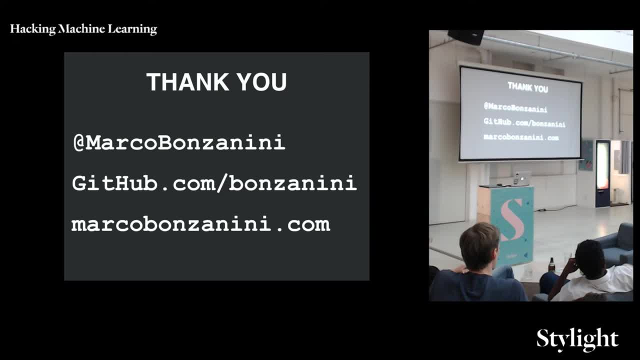 But it must depend somewhat on how many words you're training, right? I mean, it must depend somehow, like if you train on 100 million words in the text, that must somehow go into the complexity of how long it takes to train this thing. 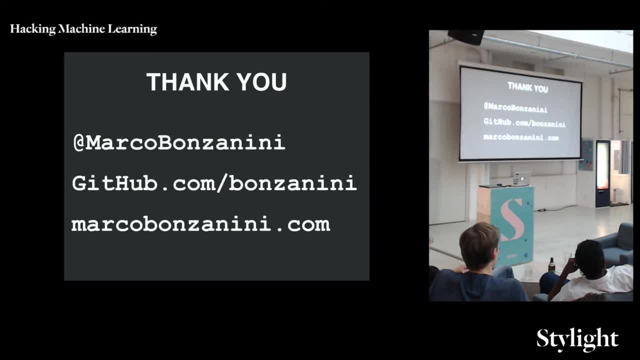 Yes, on the number of sentences really. So sentences is how you call the context. It could be sentence, It could be paragraph document. So each sentence essentially will be one of those nested loops. Oh, I see, And then the bigger picture is what dominates really. 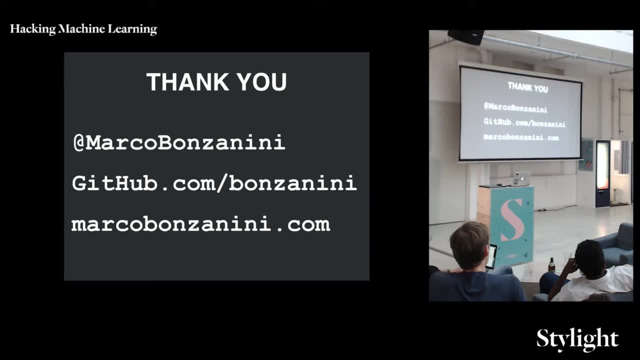 the story is anyway the size of the vocabulary. So a quick other question on priors: How do you let priors flow into this? I mean, if you know, if you have prior knowledge on, like I don't know, a beer is related to alcohol. 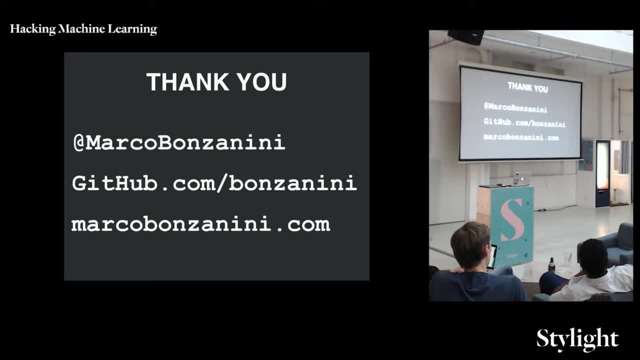 you want to put this knowledge in, rather than- I don't know- let the machine figure it out, Because you know that already. How do you let this flow into your model training? Yeah, you don't. You let the algorithm picking up the language. 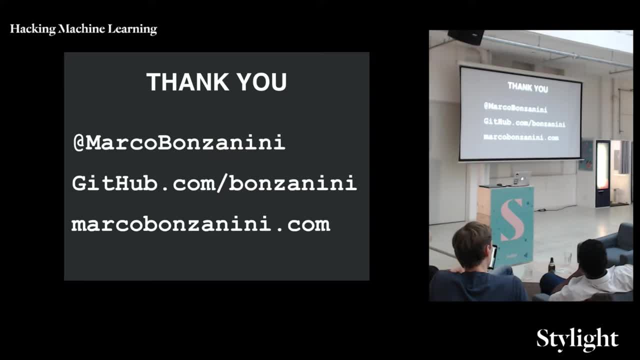 depending on how the language is used. OK, so you're limited to your training set. You cannot add priors to your model, Which is when I mentioned, when I gave you the example of pizza, and vice versa. So, essentially, your data set will. 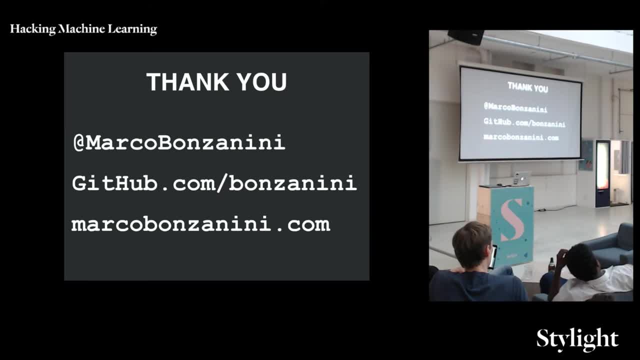 affect the quality of the vectors, of course. Usually the assumption is: with big enough data you end up with these vectors. But you can observe a lot of biases anyway. So in my example I observe bias towards American styles of beer. 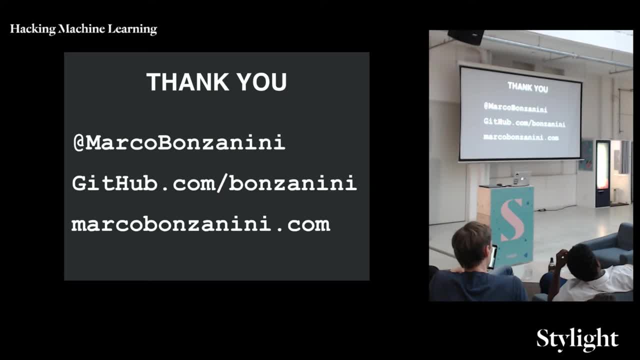 just because the data set was coming from an American website. In the Google News example you observe something a bit more disturbing because of, say, the word for Mexicans. How is the word Mexican used in American news? Usually it's about illegal immigration, right. 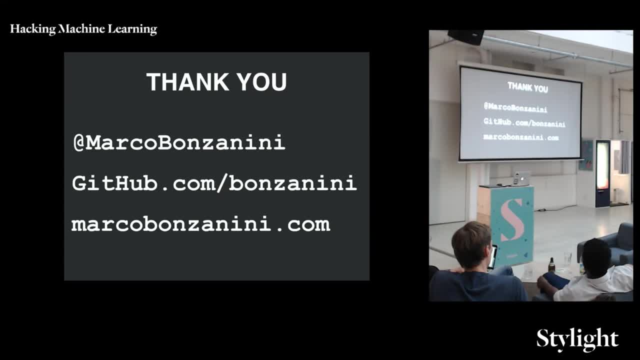 So the vector is suspiciously close to illegal immigrants, which is a strong bias. And then you observe it also with this analogy: When you do king minus man plus woman is queen. If you do programmer minus man plus woman, you expect to go back to programmer female programmer. 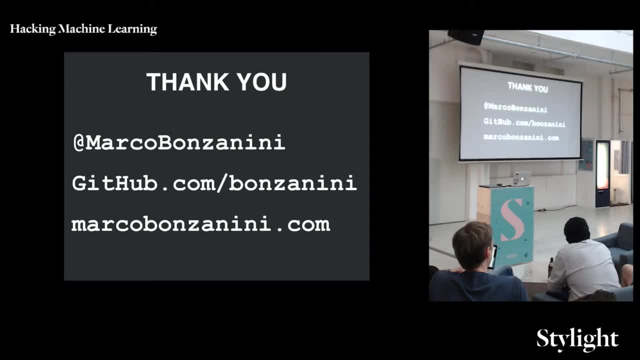 if you want, But you don't, You end up with what society thinks should be a job for women. So you have all this little kind of sexist and racist remarks because they're coming from the language itself. So language is biased And the model will pick up this bias. 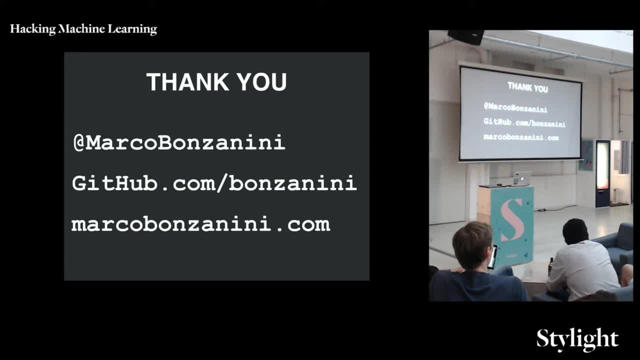 Thank you for the talk. You mentioned on your last slide a comparative model to Word2Vec glove which I think is in the theory is kind of similar but a bit different. Could you comment on the differences and pros and cons of each model, if there are? 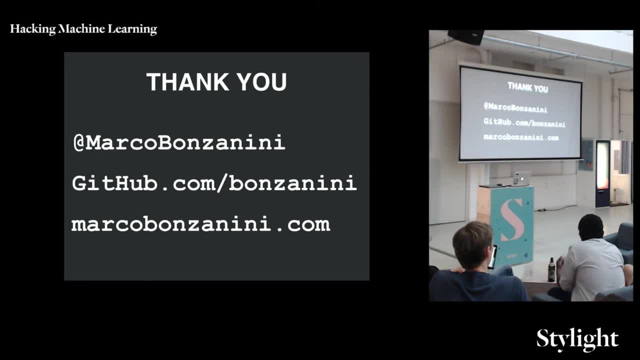 Yes, So glove versus Word2Vec. I still have to understand it. I still have to understand how they are different. They're kind of similar And for me they're very similar. Maybe I'm missing something as well, But a lot of people are asking the same question. 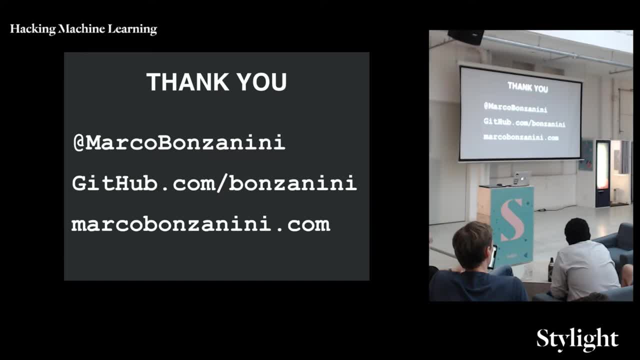 So the short answer is: I don't know. to be completely honest, And I haven't seen- apart from the guys from Stanford who are the authors of this model- I haven't seen any major improvement against Word2Vec. So I don't know. 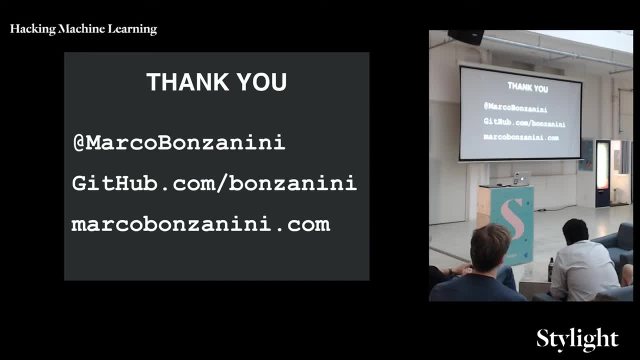 So it's there. I would like to understand it. So it's kind of a follow-up work, but I still don't know. Then one quick follow-up question back to the 300 dimensions: Is that decision for 300 more driven by the size of your data? 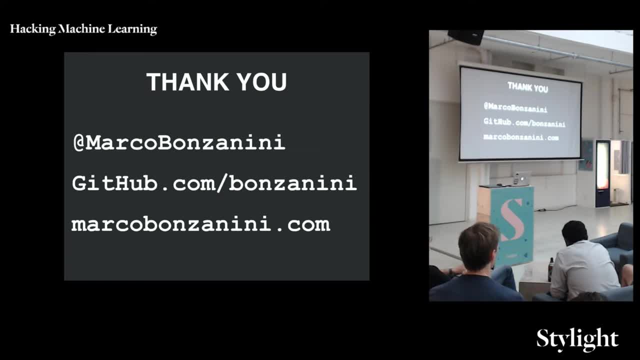 Is that or more driven by the computational time it takes for a larger number of dimensions, Or the text content is? It's just a rule of thumb, It's just empirical. That's a suggestion that was coming from the authors of the original Word2Vec paper. 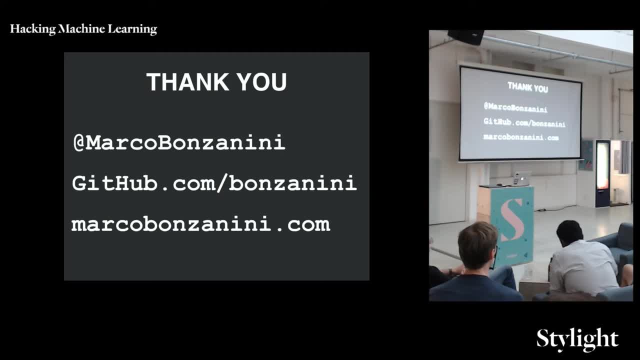 And they didn't provide any particular explanation. They said that we tried many options And the numbers I mentioned kind of make sense. So you start from there And if you like the model, you stay there. basically It's kind of small enough to be the fastest possible option. 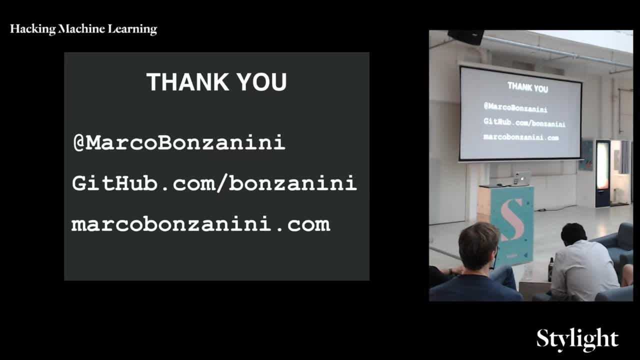 And at the same time, big enough to pick up what you want from the language. So purely empirical- I mean essentially- it goes well down to how sensitive you want to have your data set in. So if you have only one dimensions, 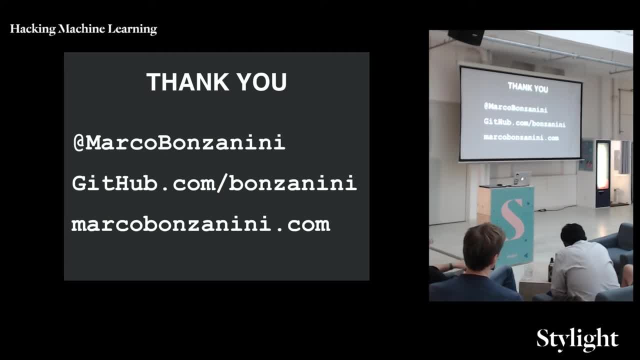 you basically have only one scale, like from cold to hot, And if you have really complicated text maybe you want to add way more, You know way, basically to compare different dimensionality of different ways, like those fours, Because eventually, if you put it in space, 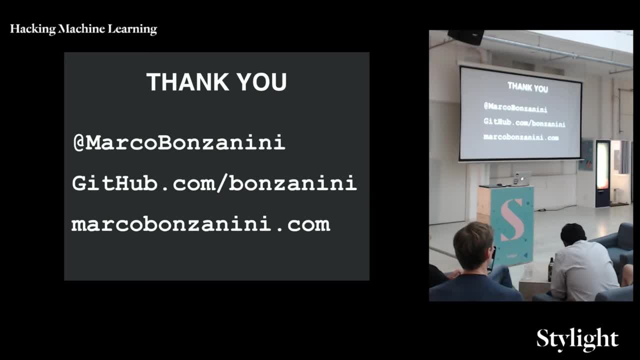 and you want to compare all this matrix multiplication that he was showing, it's basically the same. So if you want to embed more of those, you can do that, But I think there's also too much of those. So next one: Some people try to force a meaning on these dimensions. 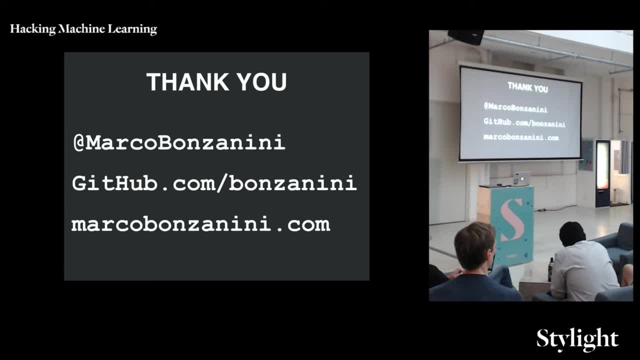 So that there's a notion. When I showed the initial example- Rome, France And so on- It's a dimension for being a city, a dimension for being a country. It's not true. So these are just dimensions. They don't mean anything in particular. 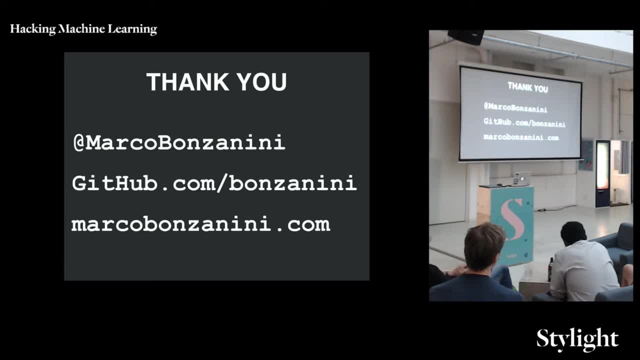 The example was just made up to the vectors And you don't find the analogies between them. So presumably you could look at the vectors and you got a sense of the doing that And I could be able to look at it And see a profile of all the interventions. 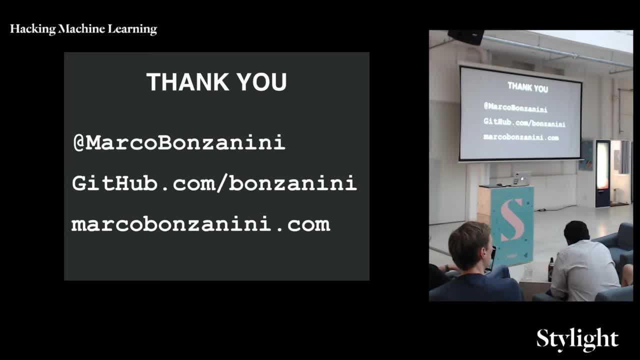 And that would give you an idea of how many you actually deal with, like the distribution of the values and the vector of interference of those dimensions. So, post-factor, you'd be able to look at and see how many you actually do in that. 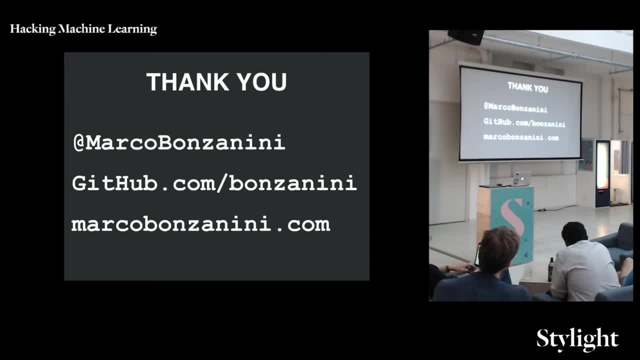 Yeah, I guess you can look at it in this way. In the case of beers, it was obvious. It was obvious to have this color dimension. But is it color or is it kind of toasted malts that are influencing the taste And of course, they influence the color as well? 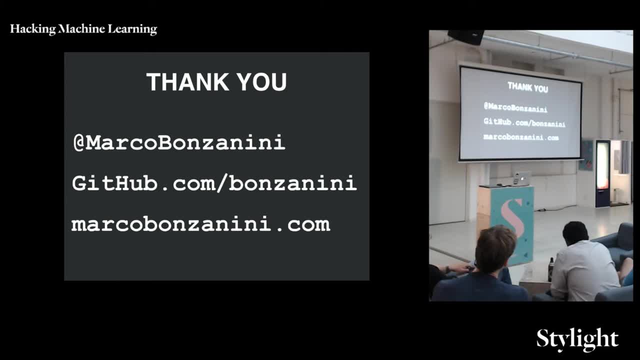 Where is the cause-effect? It was a side project for me, So just for fun, But definitely after you train you can have a look If you're planning to feed your vector to a deep neural network. anyway, how important is still the pre-processing? 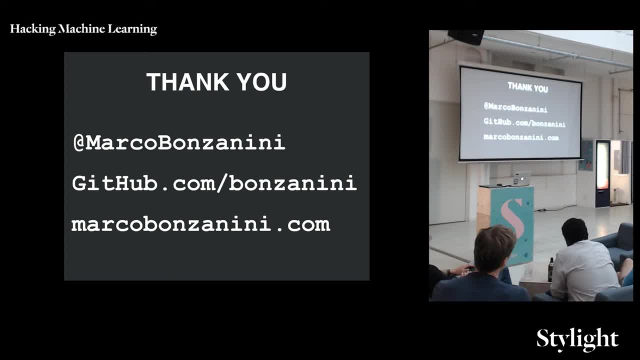 I would assume, if your data set is big enough, the vector or the deep network would already draw some conclusions that Paris is close to Rome in some way. So is that still important? I guess, with the position of the word in the sentence, you need to code that in. 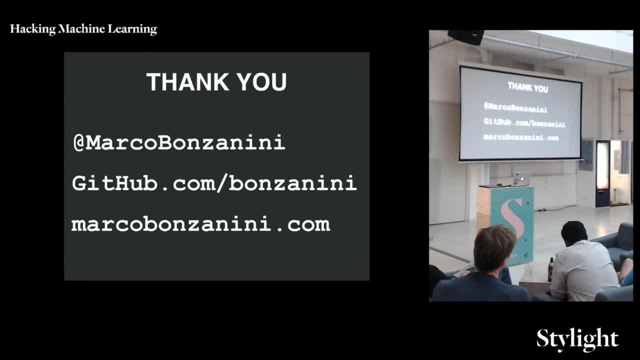 But otherwise wouldn't the deep network take that job? I guess the short answer is: it depends. The pre-processing is important to end up with high-quality vectors for words. So to perform this analysis, it's important to have high-quality vectors for words. 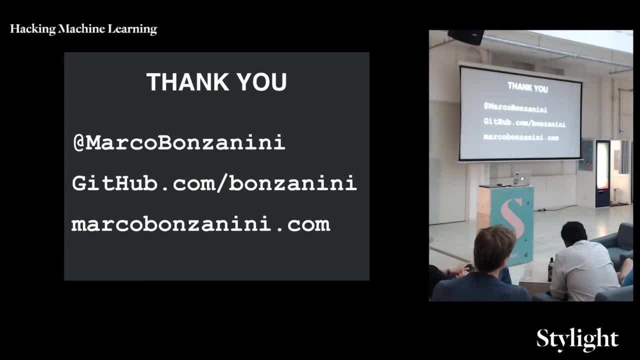 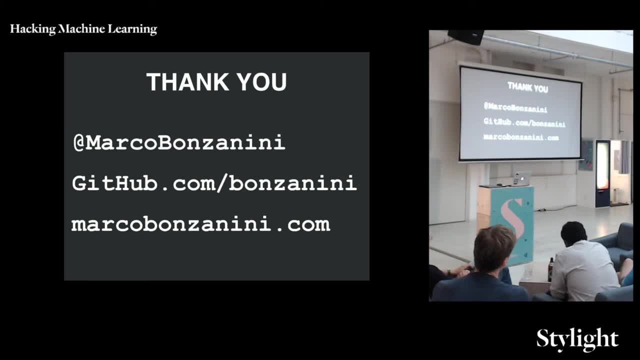 It's important to have high-quality vectors for words, And then if you fit these vectors into something else later and you have enough data, maybe that doesn't really matter. Or if you skip the vector training and you feed directly the text into whatever kind of model you have in mind. 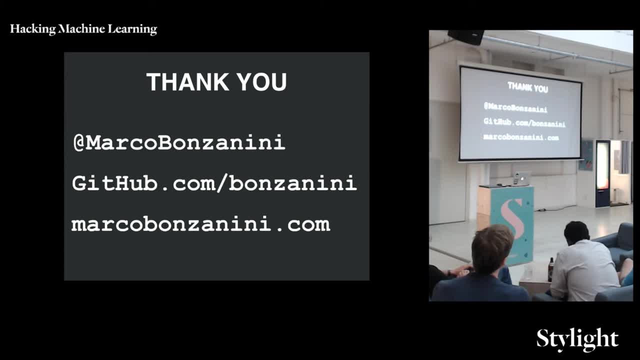 maybe doesn't matter, But what I observe is you have options essentially for pre-processing, So it matters in the sense that you have options. You can choose to do a bit of a stop Nasher removal, staming the usual suspects. You can choose to have ungrammatical sentences. 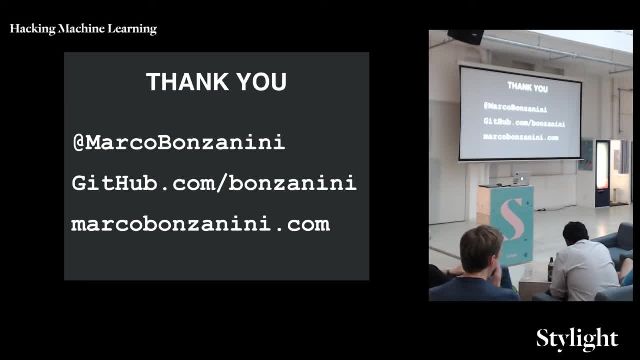 and pass only the nouns. for example, With the CV and skills example, we didn't have fluent English. We had a list of skills, So literally it was based on co-occurrences. no grammar picked up whatsoever, So it matters from this point of view. 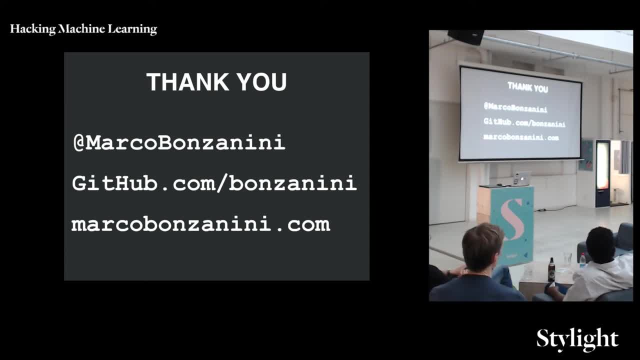 Then whether it will improve the overall quality, that's to be tested on your data. I would say: Is there a specific procedure you would suggest for a chatbot? I don't know. I don't know. I haven't developed chatbots. 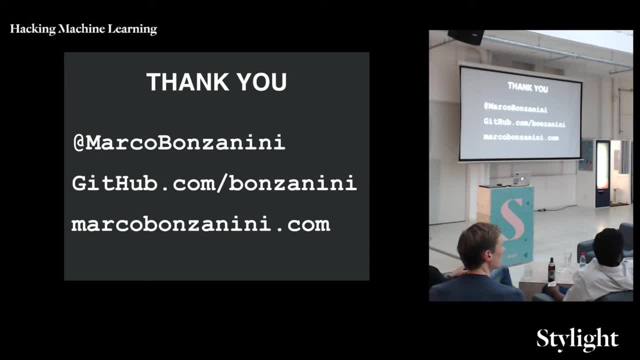 I don't know, Hi. Thanks for the talk. Do the vectors come out of the Word2Vec algorithm normalized, so do they have the same length or do they have different lengths? Are the vectors, Sorry, Normalized Or are they different lengths? the vectors? 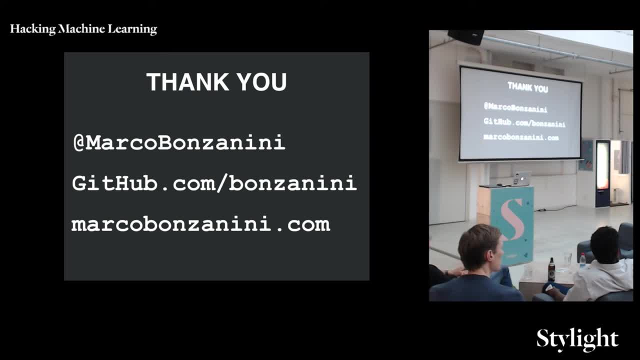 No, the number of dimensions is fixed. No, but the length of the vector, the norm. Oh yes, So all the dimensions are essentially between 0 and 1.. But do they have the same length? So if you have two words, do they? have the same length the vector, Or does it depend? So what people do, usually they merge. So if you want to model a phrase, you merge it. You kind of create a special token of Word1 underscore Word2.. Is that what you're asking? 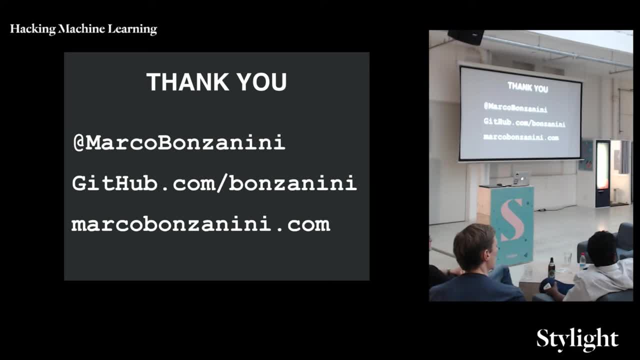 No, I guess. I mean, if you look at the mathematical object of a vector, it has a direction and a length, And are these vectors all the same length and just different directions, or are they different lengths and different directions? I noticed that when people try to compute the similarity between 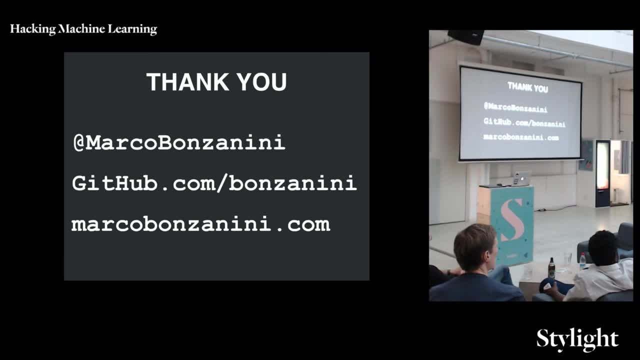 let's say, first normalize the vectors and then do it. So I guess they are not normalized before. I'm not sure I understand the question. So maybe we chat later. Yeah, OK, That's a question, Maybe last one. 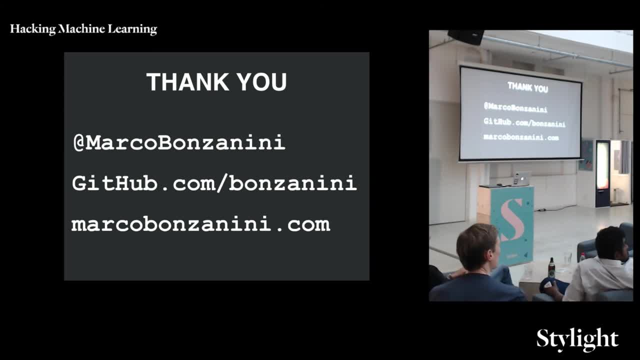 No, OK, This one on the back. I can see you. You're like behind the wall. I'm bringing that. I have three questions for you. So how big was the memory footprint in your RAM So while you were computing with that metrics? 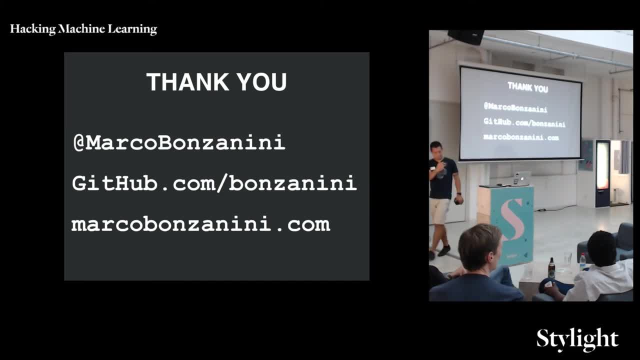 The memory footprint. Yep, I wasn't checking the memory footprint. It was fitting in memory on my laptop. The data set was the bigger one was about one gigabyte, so nothing huge. The output is about 150 megabytes from one gigabyte of text. 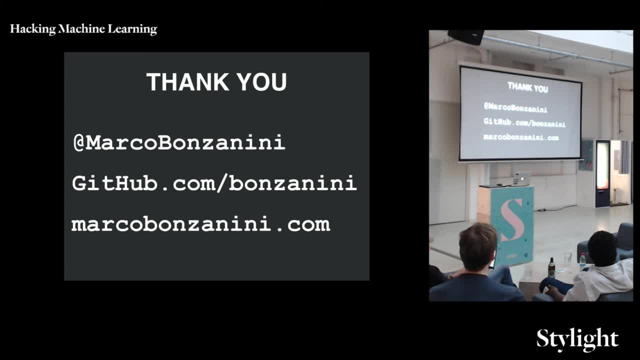 to 150 megabytes over, So it's a lot of data. OK, So when you're saying the output, so were you able to save that output for some later computations also? I'm assuming Can't hear you, I'm asking you so when you computed that metrics? 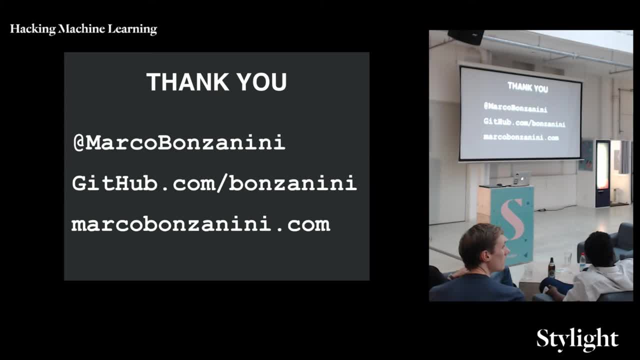 were you able to save it offline, For example. you don't have to compute next time when you were, let's say, planning to play with the data. So, first thing, there is no metrics computed, They're just vectors, And you can persist the model and then 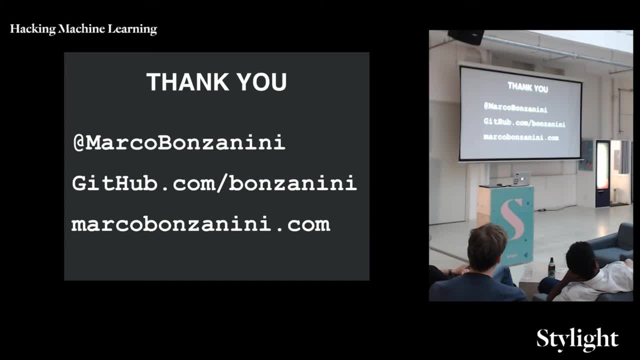 continue the training later. OK, So you can add more data later on and it will, in theory, improve your vector representation. Thank you, It answered my third question. yeah, Can I retrain? Yes, I can retrain. 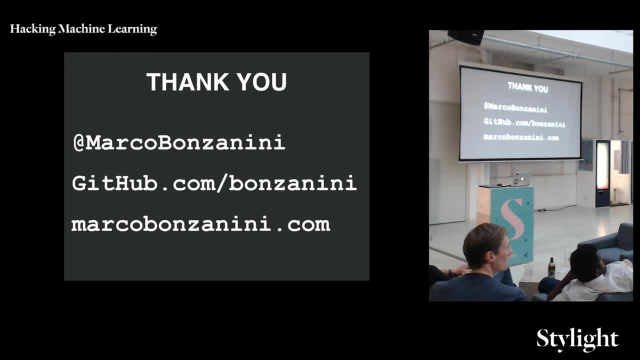 Awesome, The last, last one. no, OK, Here's the winner, And after we're having a break. So I'm interested in the work to sentence stuff, Sentence to vector, you know? Yes, Do you have to predefine, like, the number of words? 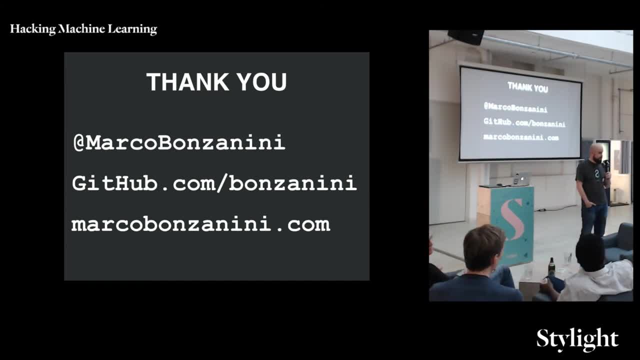 in a sentence you want to match, like with, for example, a wheat stout, or actually two words, or is it just OK? So the notion of sentence as described in these papers is just a piece of text, So it could be an actual sentence in English. 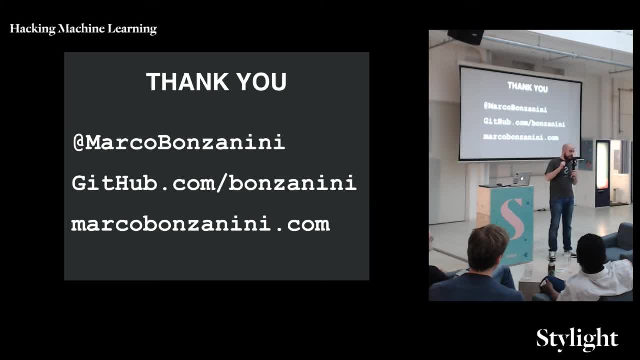 or it could be a paragraph, whatever you want, And you can choose a size for a window. so five words before and after the focus words. Or you can say let's use the whole sentence, And usually I use the whole sentence. 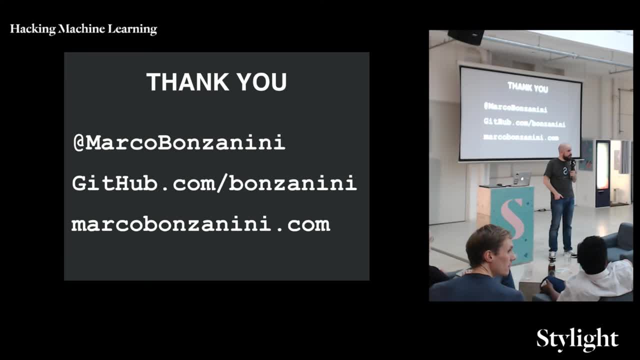 unless I have a very, very huge difference. But how is the sentence defined? Is it like with a dot, like from one dot to the next dot? Or how do you define a sentence? It's up to you in how you preprocess. 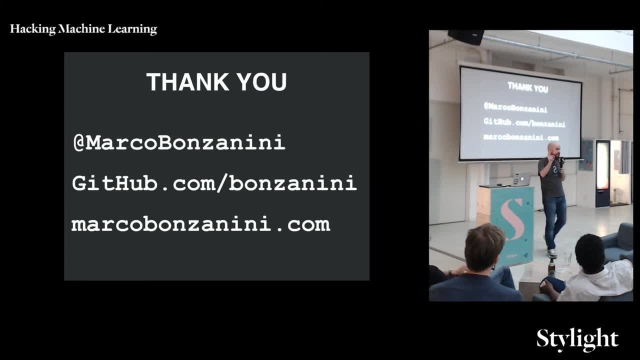 For the CV example. the sentence was an experience in your CV, So it was not an actual sentence Review. I was just using, if I remember well, this DNLTK tokenizer out of the box to split sentences. It's up to you how you define it. 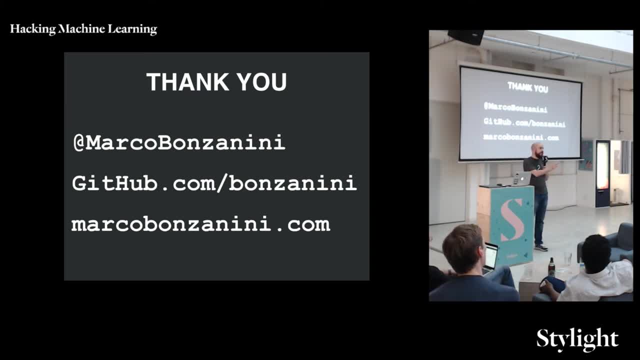 But you need to feed the sentences. so a generator of sentences to define it on your own, And how you do it is up to you. You can pass the whole document if you want. OK, thank you. OK, thank you again for awesome talk. 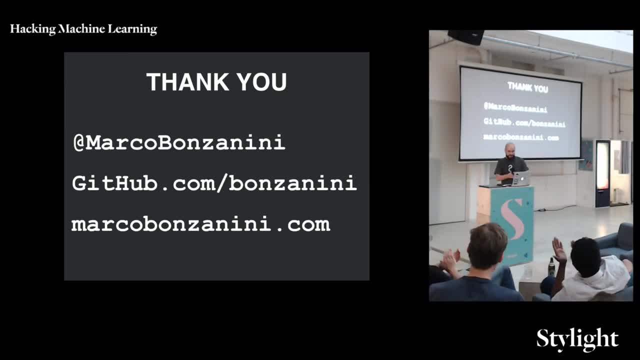 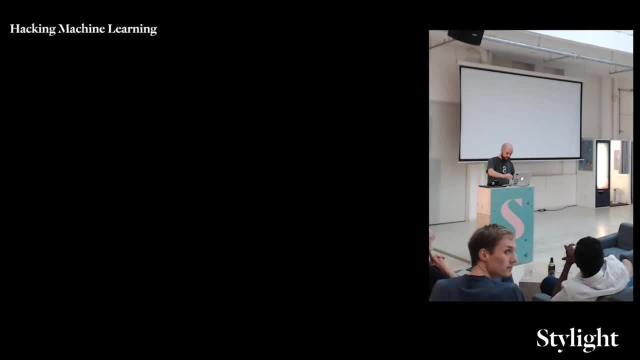 And awesome Q&A session, Thank you. Now we're having like a break of five minutes and continue with the second speaker. So yep, And there'll be a URL on the screen For anyone who wants to follow along on their laptop.